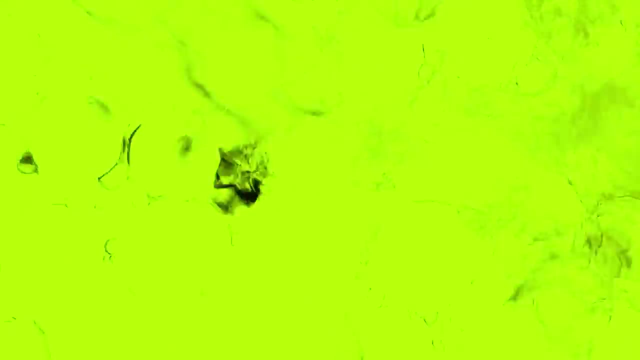 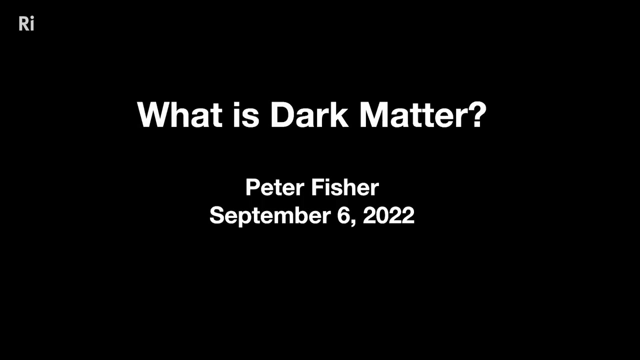 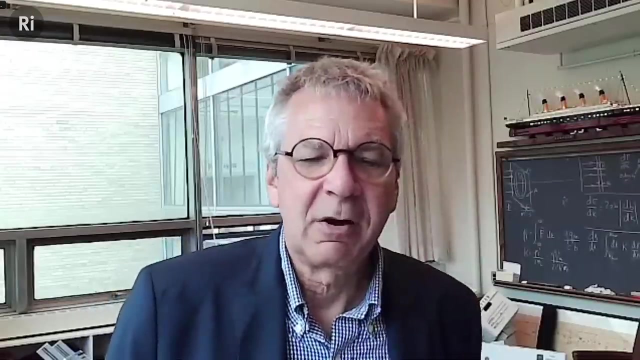 Yes, hello. Thank you, Lisa. And our topic for tonight is- you can, as you heard- is: what is dark matter? I'll give you kind of the main bullet points, which are: we know dark matter exists because of the way things are shaped in our universe, but we don't know what dark matter. 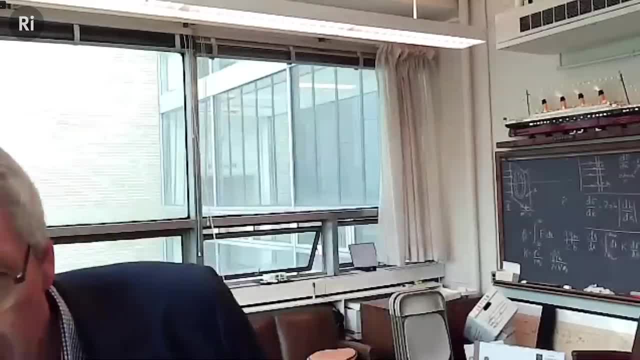 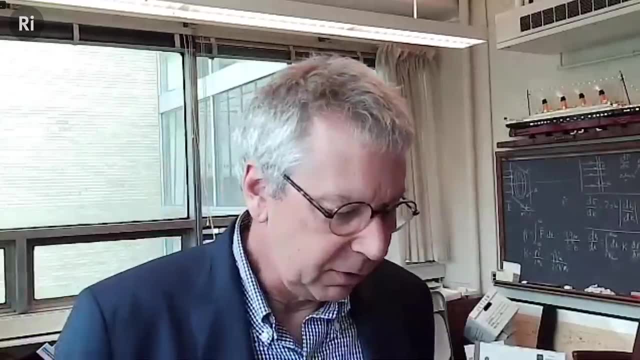 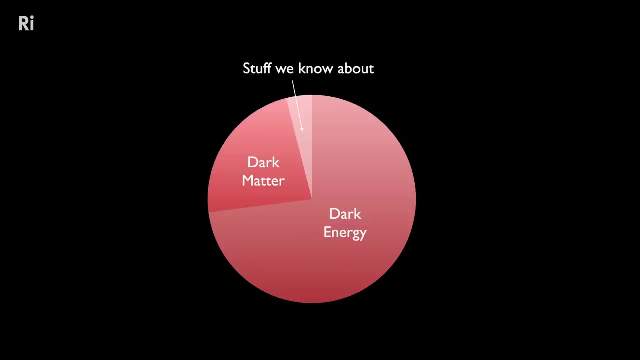 actually is. So the rest of the talk in my book, which I'll show you here, will flesh out and elucidate those two ideas. So you should be seeing a slide. that's a pie chart and it shows how the energy and matter in our universe is apportioned according to the best measurements we've been. 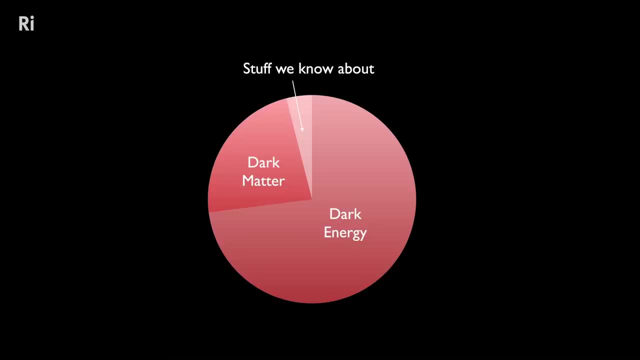 able to make both in particle physics and astronomy, And there's some kind of an odd history to this slide. Over the last hundred years, particle physics, which started just about 120 years ago, evolved so that by the early 1990s we had a very 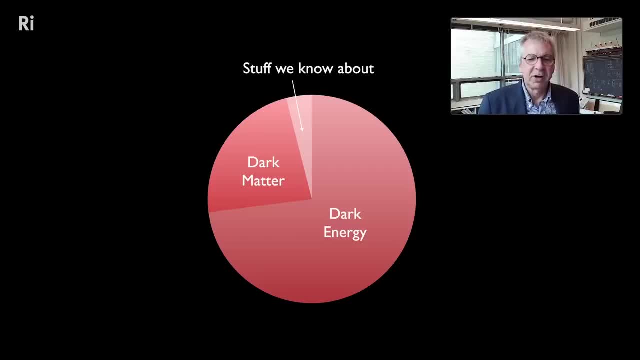 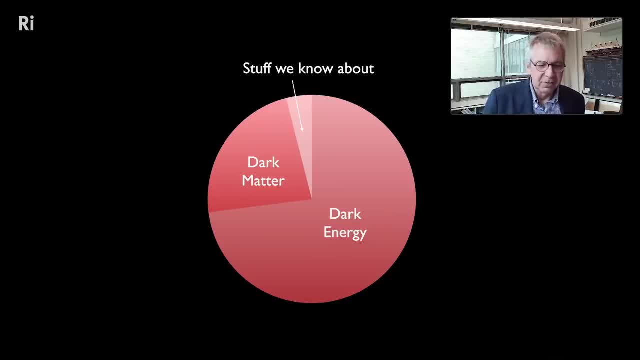 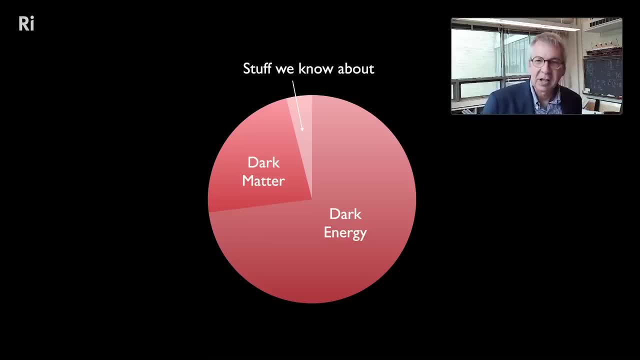 became available to make microwaves and accelerators, And there was an explosion in understanding of particle physics that lasted until well, until the present day, but really reached its zenith in the 1990s, And so coming into the early 1990s. 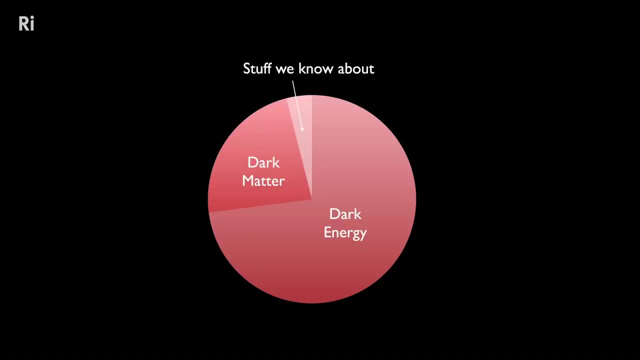 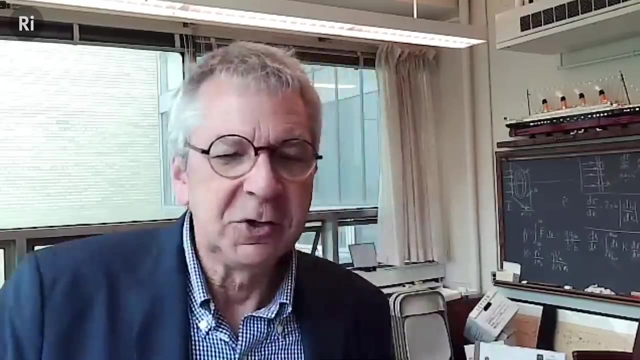 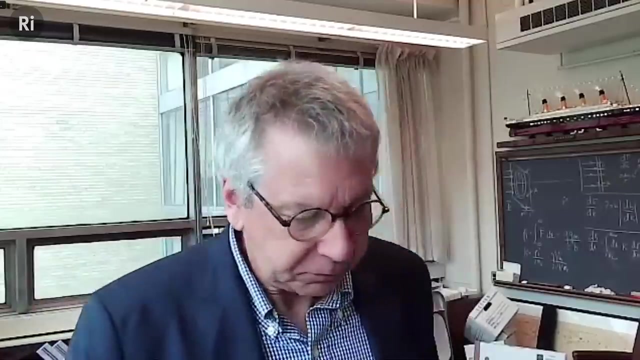 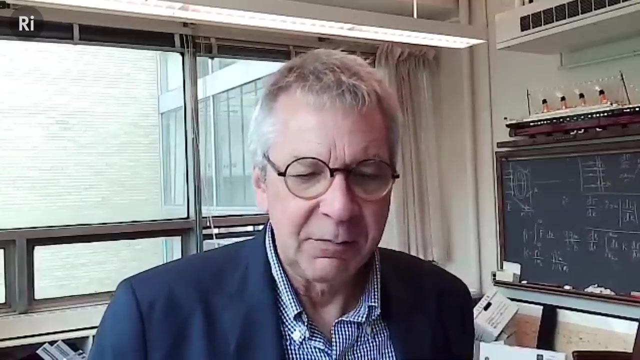 physicists thought that we really understood the totality of matter or energy in the universe. And we talk about matter, energy interchangeably, because E equals MC, squared, as Einstein told us, And so we can just talk about one or the other. Along the same time, astronomers were developing. 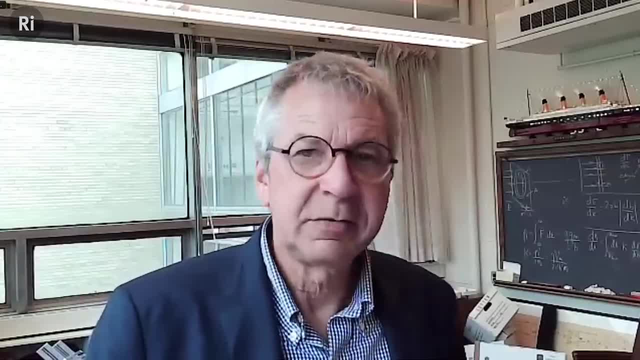 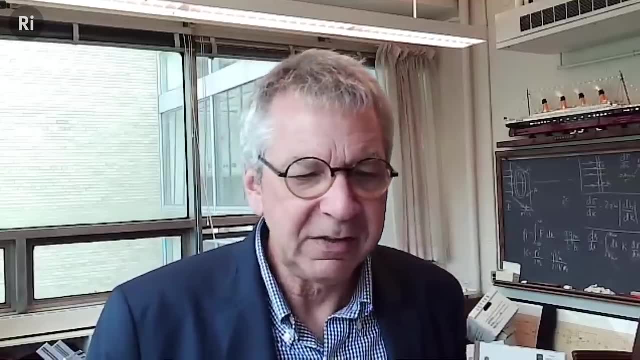 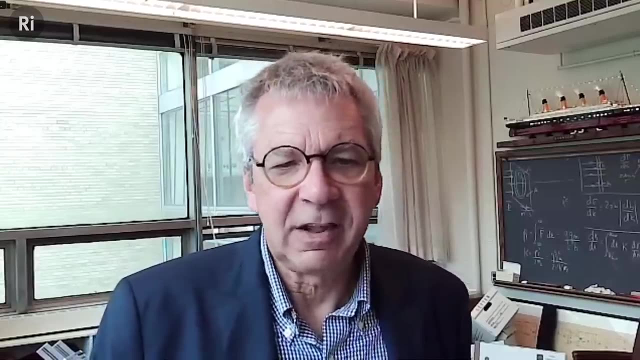 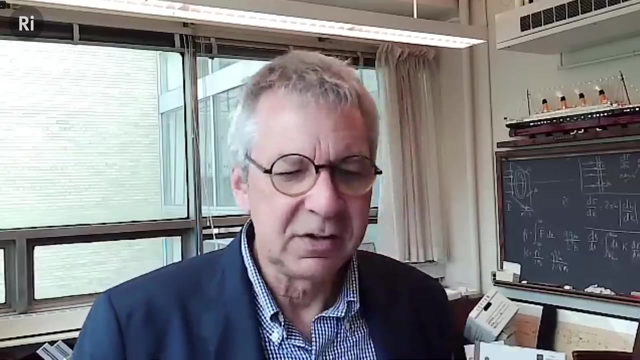 bigger and better telescopes and more advanced observing techniques, And And so, in the 1920s, astronomers discerned that the fuzzy, star-like objects that they called nebula, which means fuzzy or foggy, were actually distant galaxies like the Milky Way, with hundreds of thousands, hundreds of millions or trillions of stars. I'm sorry. 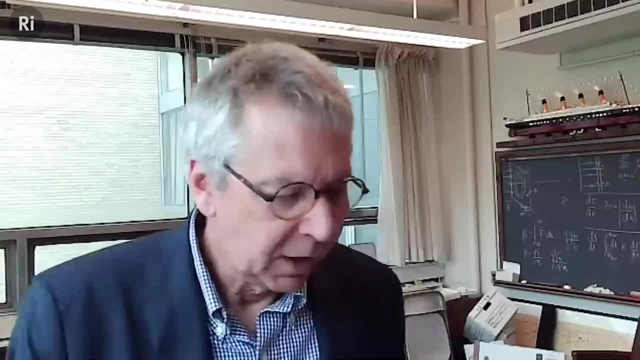 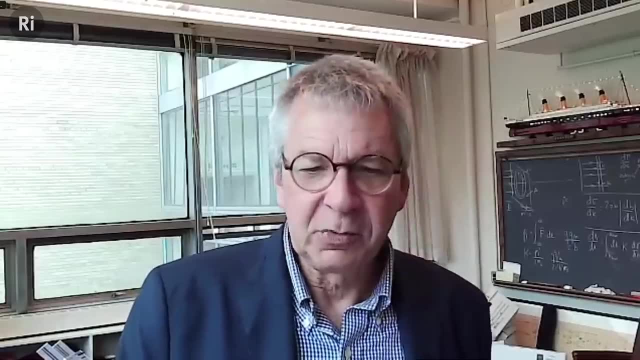 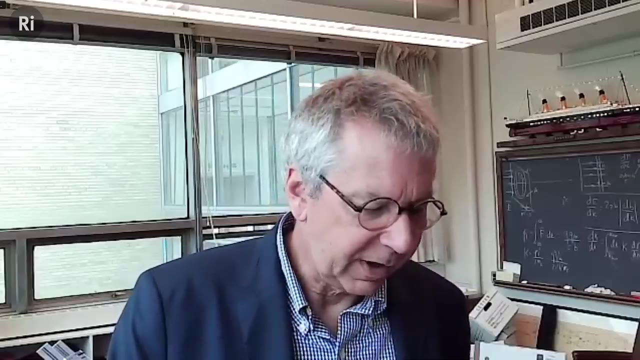 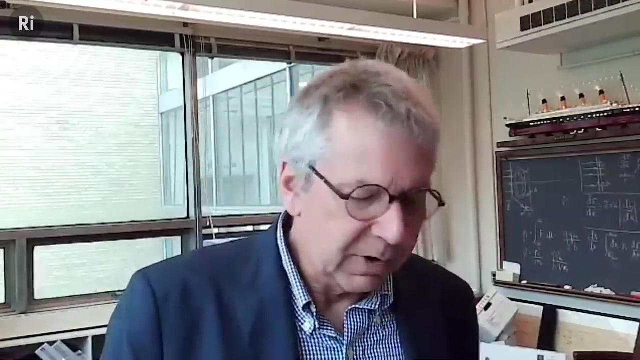 trillions of stars in them gravitationally bound, And very shortly after that there were a series of observations that indicated those stars were moving too fast to account for the matter in the galaxy, And I'll talk about that more later. As observational techniques improved, the acceleration of the universe became clearer. 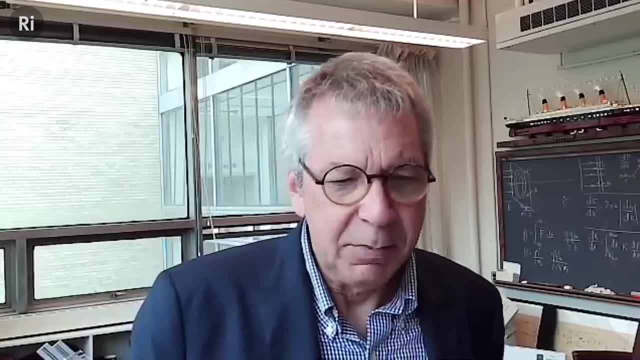 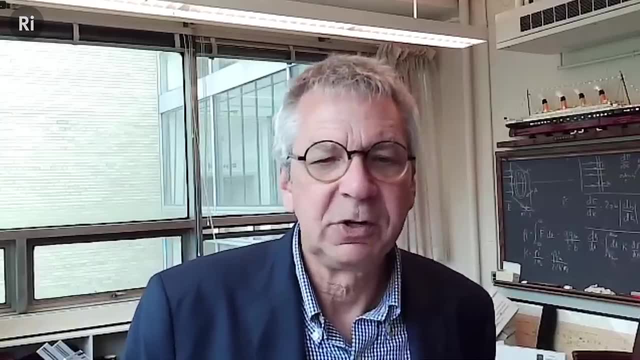 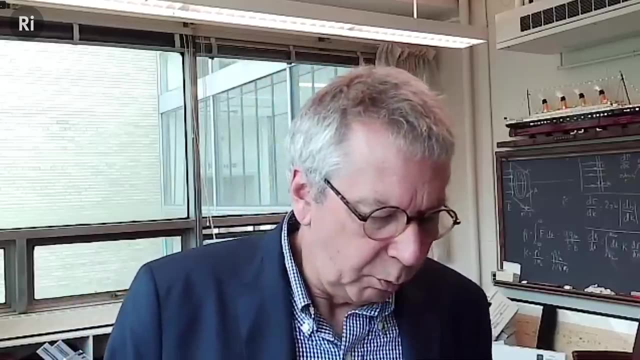 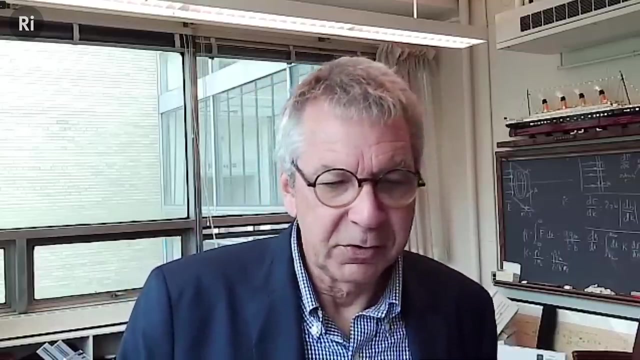 And the acceleration of the universe is actually space-time getting bigger, which means that those galaxies are seem to be moving apart with a velocity that's proportional to the distance between them. This was quite surprising, And measurements of this acceleration, which is also called the Hubble parameter, improved. 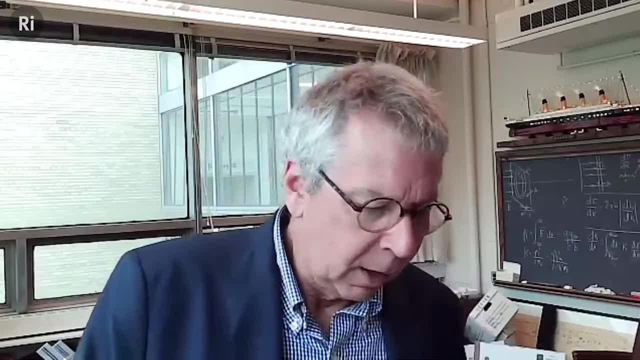 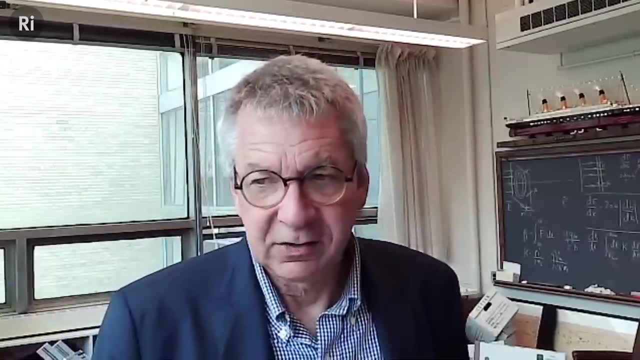 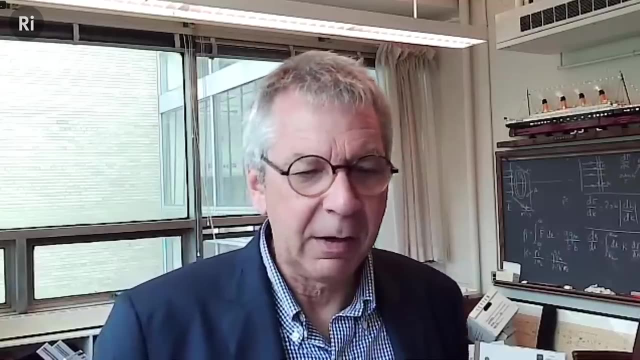 through the 50s, 60s and 70s. By the mid-1980s, astronomers had developed techniques using exploding stars called supernovae, And they used supernovae to be able to look really halfway across the galaxy, or halfway. 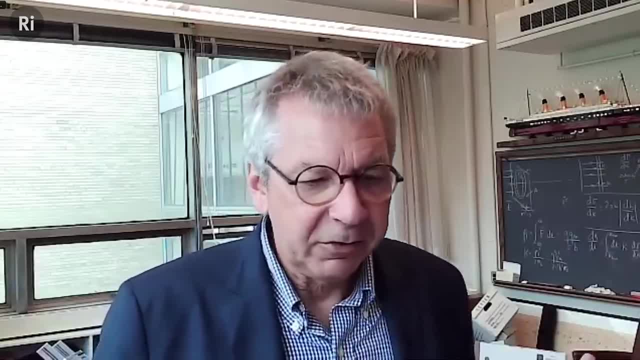 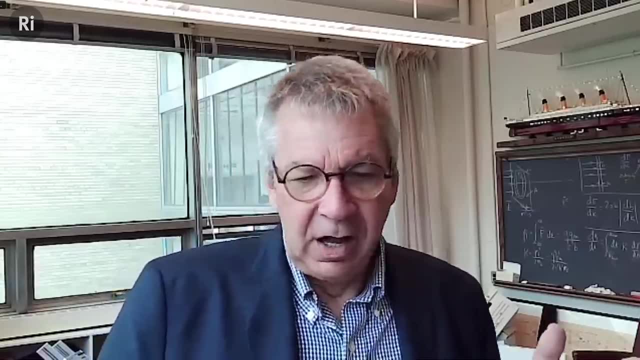 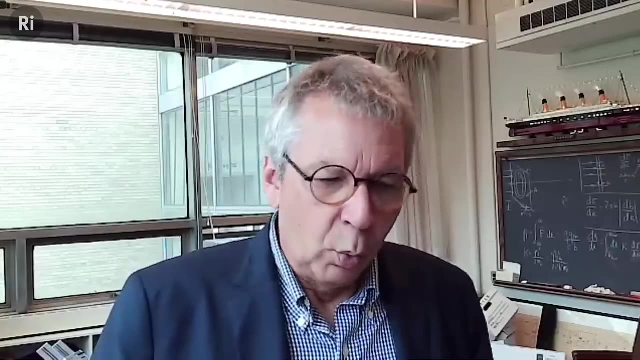 back in time And remember. light travels at a fixed velocity. So when an astronomer sees light from a distant star in their telescope, what they're actually looking at is light that was emitted by that star hundreds of millions or billions of years before. 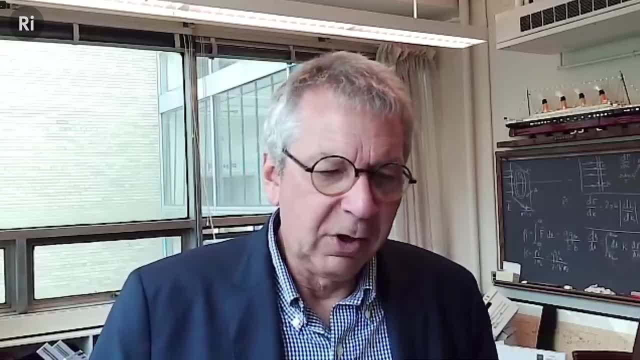 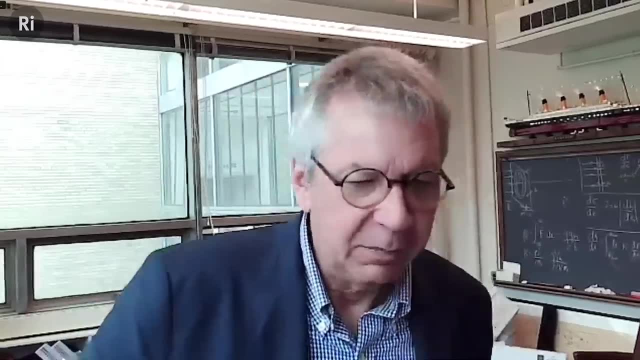 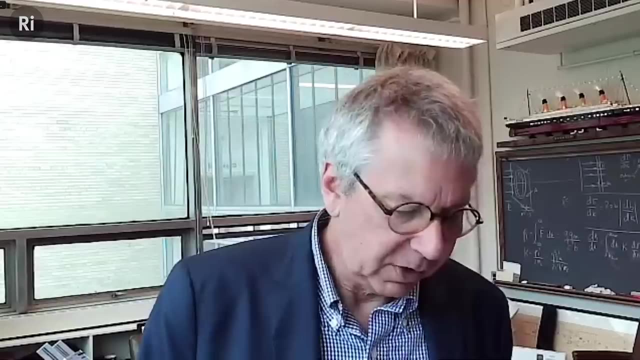 And so when an astronomer looks at a distant supernova, they're actually looking back in time at how the universe was, for example, if it's halfway across the galaxy, halfway across the universe, when the universe is half as old as it was now. 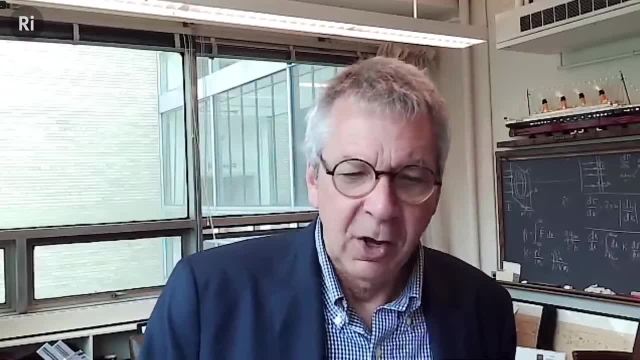 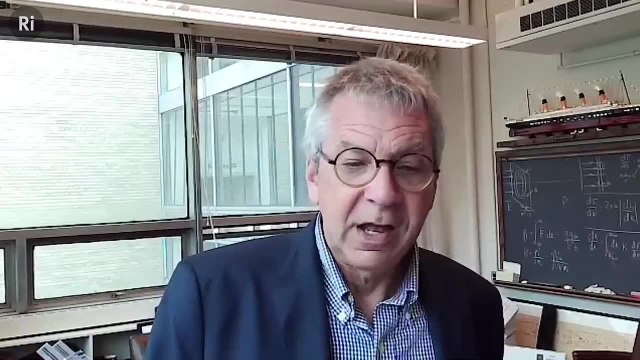 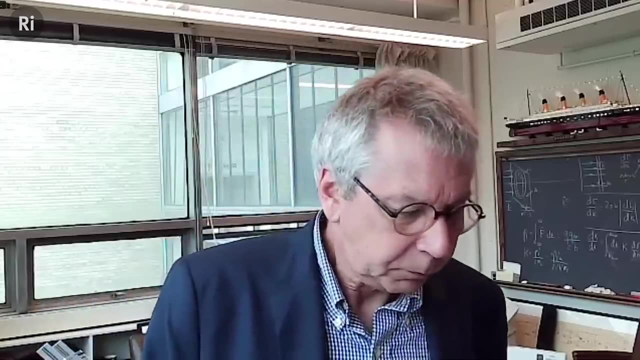 And so being able to look halfway across the universe at these supernovas showed that not only was the universe accelerating, expanded, but that expansion was was was accelerating, And that gave rise to dark matter's cousin, dark energy. So the two discoveries of dark energy and dark matter, one of which I'll talk about, 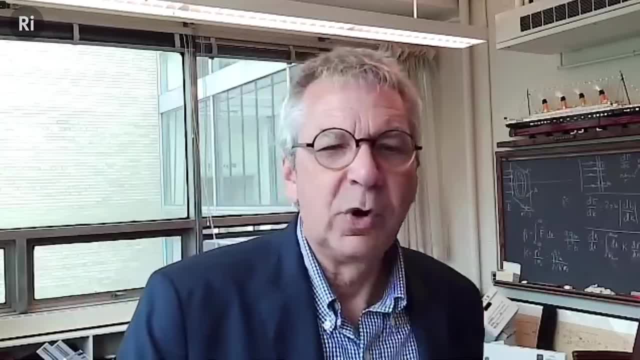 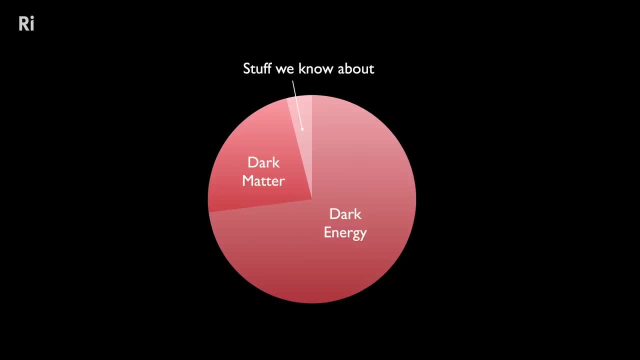 tonight told physicists and astronomers, really, and we can have the pie chart, that the stuff we know about, which I've labeled stuff we know about, which are the atoms and molecules and photons and all the particles we made in accelerators, is really only four. 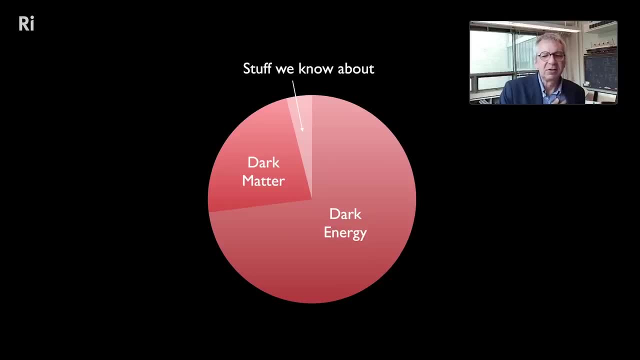 percent of the matter energy in the universe. Twenty-three percent is dark matter and about 73 percent is dark energy. So it's a little ironic that two fields, closely related but distinct, pursued roughly parallel courses for a hundred years, and one informed the other that it had only done four percent. 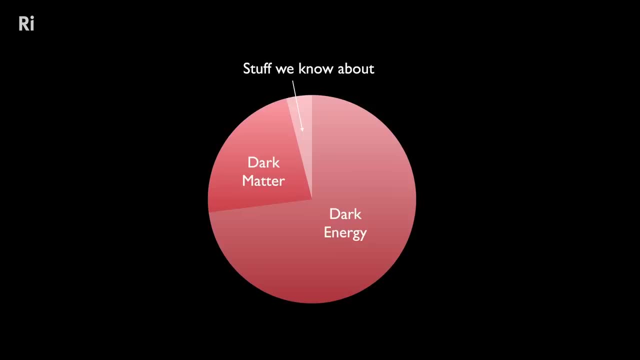 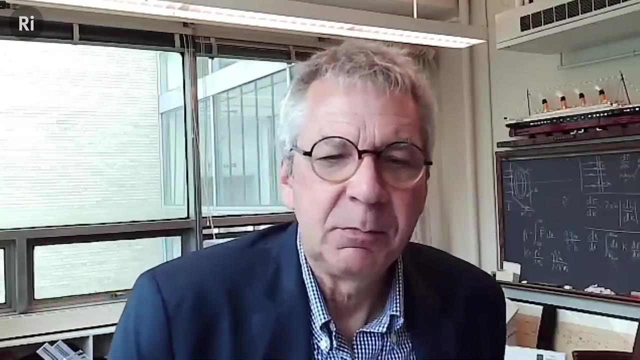 of the work. Can we stop sharing for a second? Okay, Let's stop sharing for a second. So tonight, what I want to tell you about is a little bit about dark energy, because it's a cousin of dark matter, and I want to tell you a little bit about it so that it's 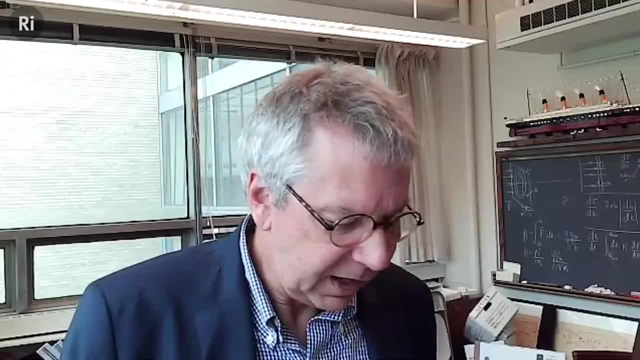 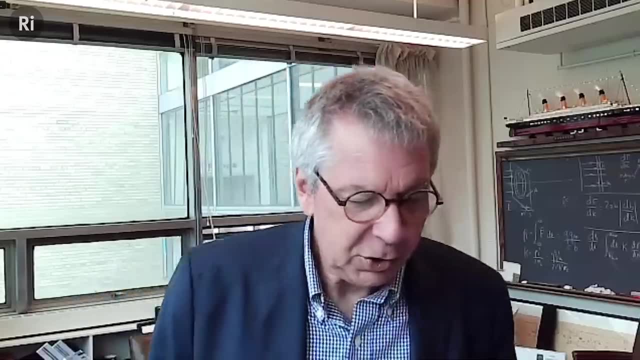 clear that it's really a different phenomenon and a whole different story, a very interesting one, but not one we'll talk about tonight. Then I want to show you two pictures from two very different telescopes and talk about how dark matter makes those pictures look the way they are. 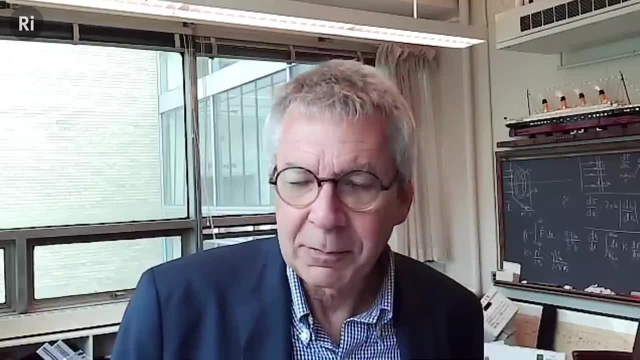 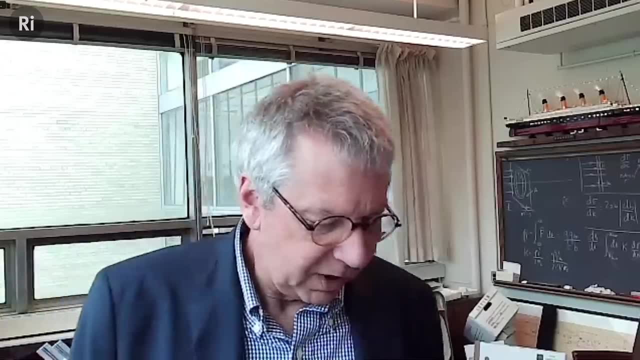 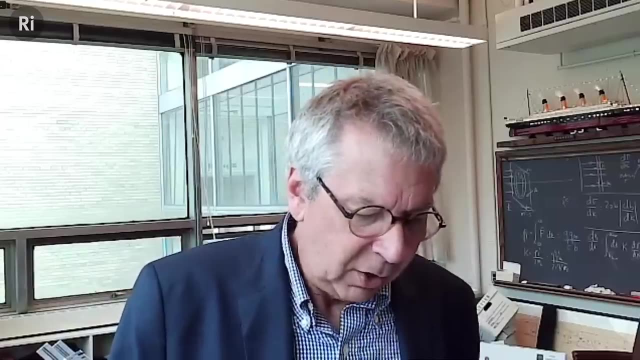 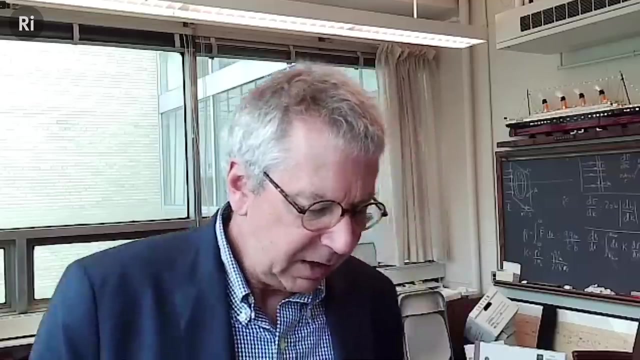 Because a major theme for this talk is how dark matter makes the universe appear the way it is Now. I want to give, then, three or four examples of different phenomenon that have been observed by astronomers, showing very different mechanisms by which the dark matter has shaped our universe. 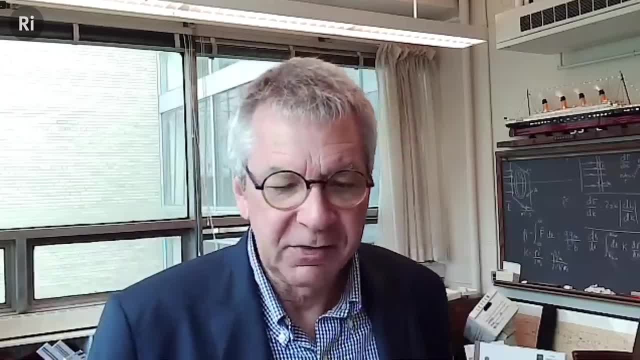 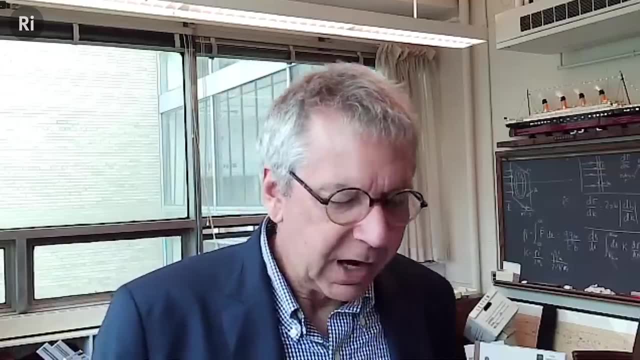 and then move on to the question of what is our current picture of the universe. What is our current picture of the universe? What is our current picture of the universe? What particles do we know about and why are none of them? the dark matter particle. 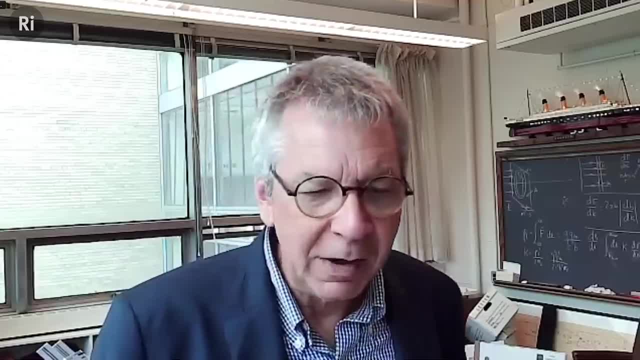 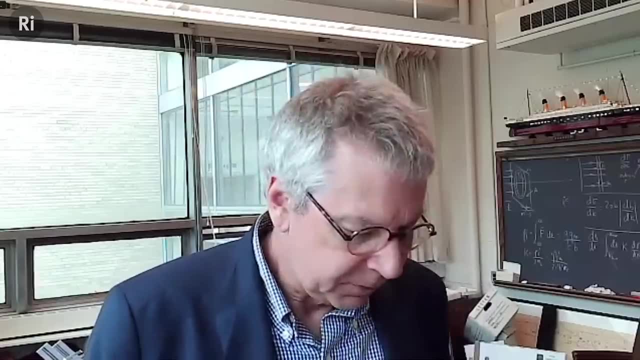 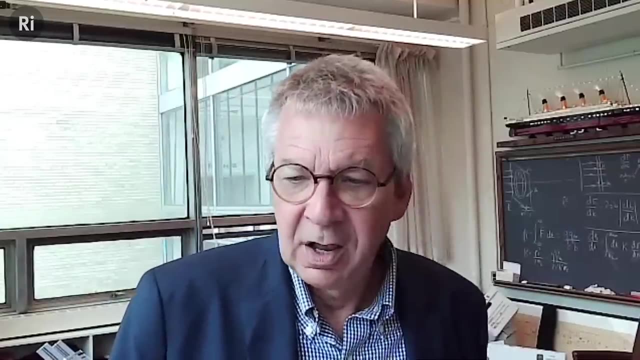 And then I want to give you three examples- the three most popular examples- of what dark matter could be and say a little bit about how we search for them. So this is something I've been involved with for about 35 years. I worked on one of the very first dark matter experiments as a graduate student and had 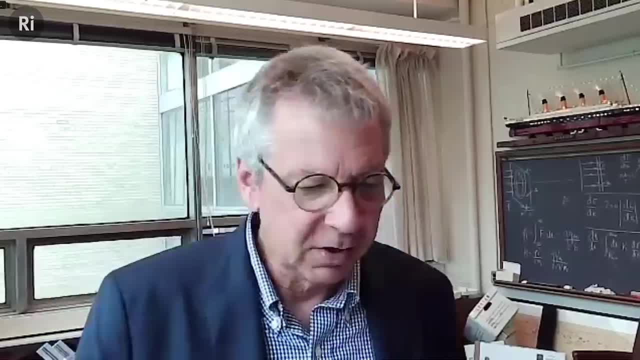 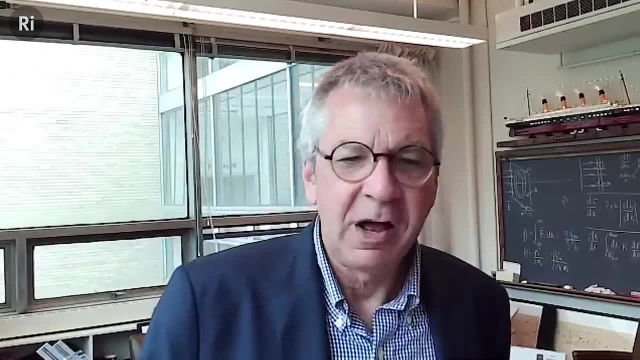 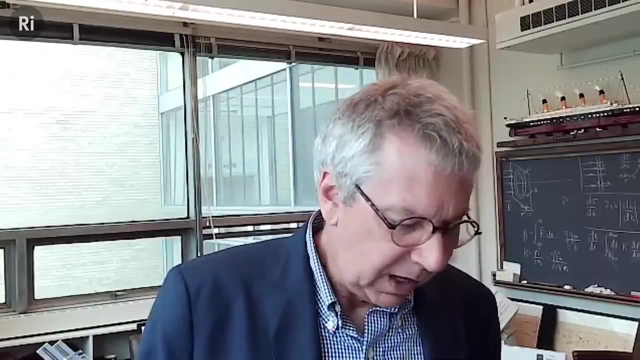 a really marvelous experience. I had a marvelous adventure, worked with many wonderful people and done a lot of interesting things. I'll tell you a little bit about them, But I have not found dark matter and I'll give a perspective on the future of this endeavor. 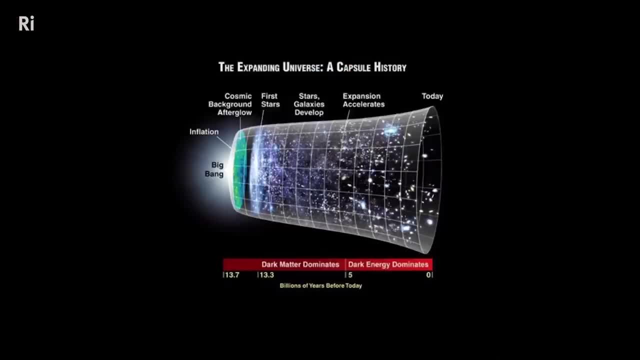 in a few minutes. What's shown here is the universe evolving from left to right. You can see Big Bang labeled there. in the background, You can see the light glow of the star of the universe And then, as time passes- and the Big Bang was 13.7 billion years ago, as indicated on- 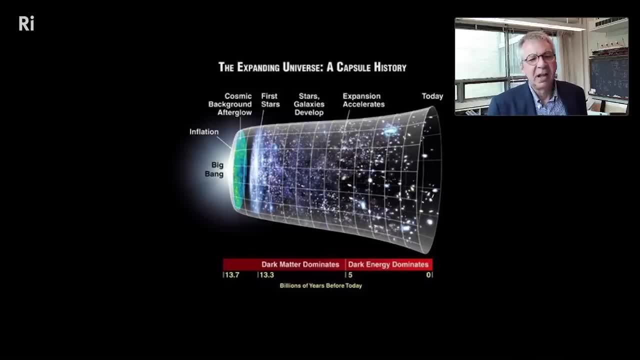 the bottom the universe expanded and that's indicated by the way the disk that represents the universe gets larger. So there was an initial very rapid expansion labeled inflation. That's a theory by my colleague Here at MIT, Alan Guth, And that's an entirely different and no less fascinating story. 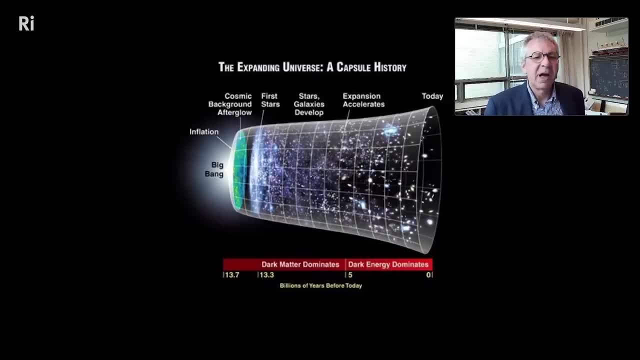 And then one of the first things that happens in the universe is the cosmic background afterglow, And I'll tell you what that is in a couple of minutes. But after that happened you can see the universe gets bigger only very slowly, going from left. 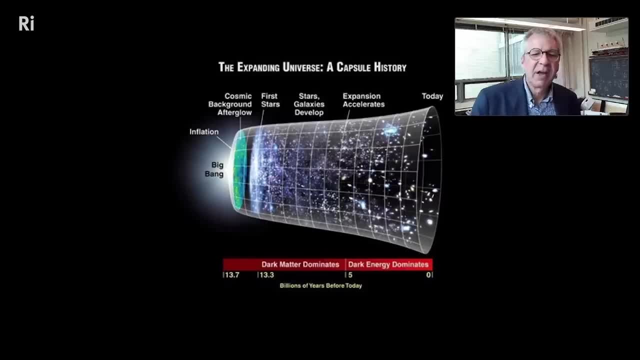 to right And that's indicated sort of by the diameter of that trumpet shape And you can see where the first stars, stars and galaxies develop. And then you can see, a little bit more than halfway down, that the radius of the universe starts getting bigger, faster. 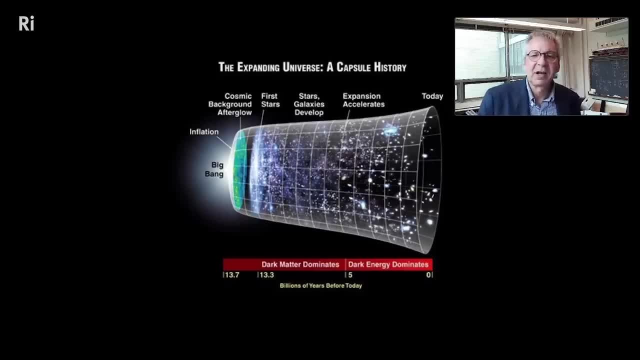 It's starting to curve a little bit, which means that it's accelerating And that's really the action of dark energy. So dark energy is somewhat mysterious. There's no quantum mechanical theory of dark energy that's been shown to be correct. But it fits very naturally into Einstein's theory of gravity, which is not a quantum. 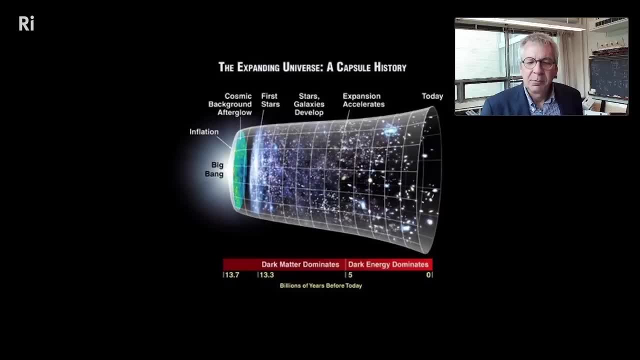 mechanical theory. In fact, it's just one number that appears in Einstein's theory. You put that in, you measure that number and you can explain how the universe is expanding and that expansion is accelerating. And, as I mentioned before, that acceleration was discerned by looking at very distant supernova. 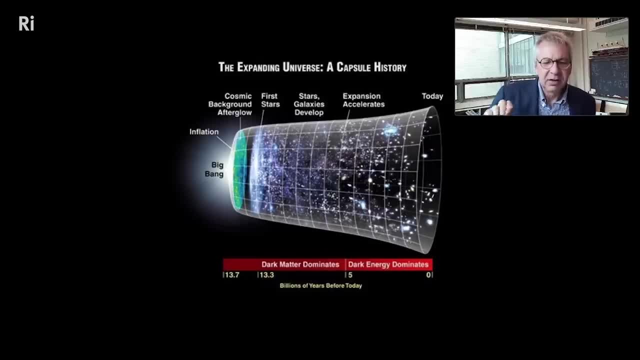 whose energy output you can calculate, because they're a special kind of supernova And that tells you how bright they are. You can measure their redshift, which is a technique astronomers have for measuring how fast something is moving away from you, And compare that velocity with the distance. 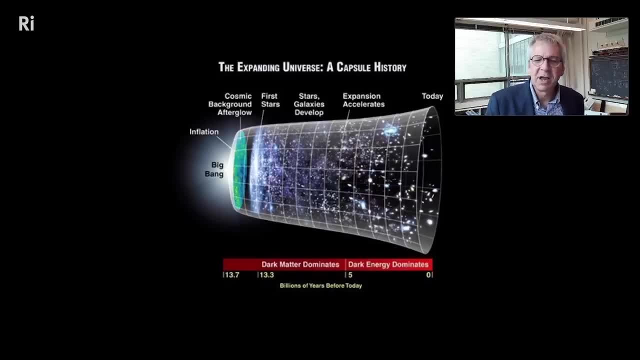 And that's what you get. You can get the acceleration of the expanding universe. What this says is that every square centimeter of our universe is filled with something called dark energy, that is, a substance that has negative pressure, And that negative pressure, somewhat contradictory, makes the universe expand. 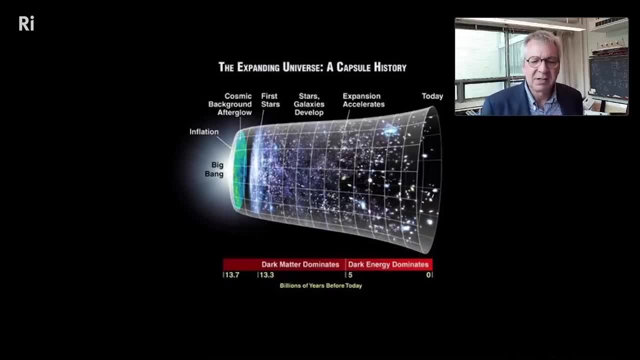 It drives an ever-increasing…. Well, I know at least a few of you are in finance and so you can think of dark energy as compound interest on space-time, And you all know that compound interest. it starts out small but you give it enough time. 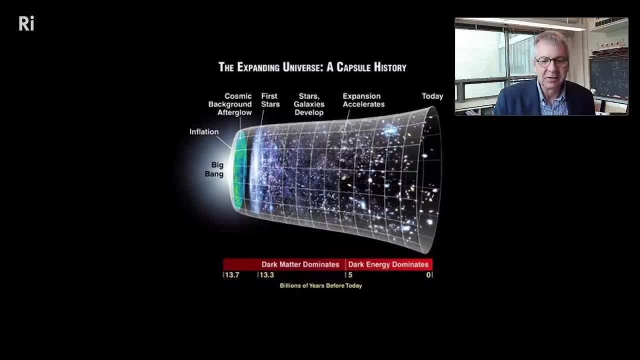 and it gets big. That's how university endowments work in the universe. That's how you do it. That's how you do it in the United States, because universities can be around forever. It's the same thing. The universe right now gets about 7% larger. 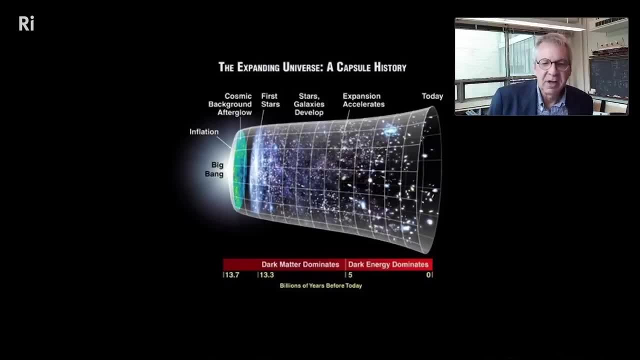 Space-time expands by about 7% per billion years, And so for that whole first 8 billion years you didn't notice the universe doing anything except sort of expanding linearly with time. And it's only now. It's only now. 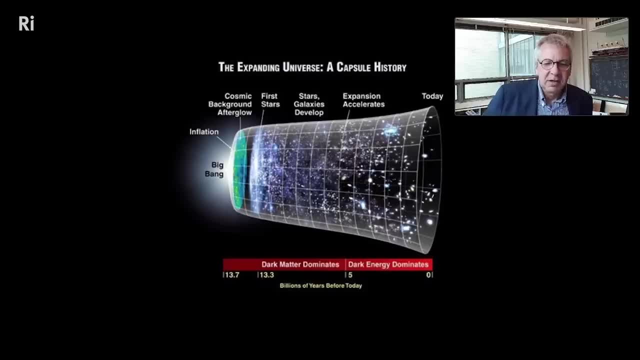 In the last 5 billion years the quadratic part, or the curvy part of the compound interest on the space-time of our universe is really starting to make the universe expand. So dark energy in a certain way shapes our universe as well. but it's a little bit boring. 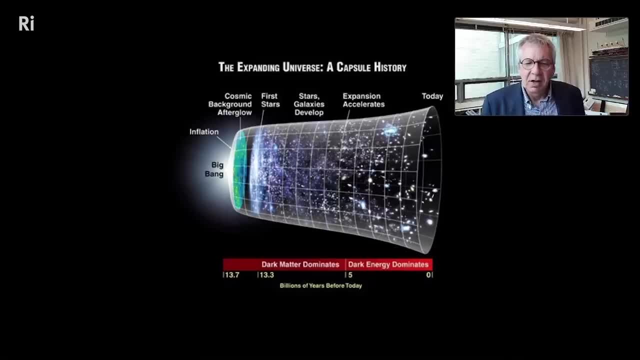 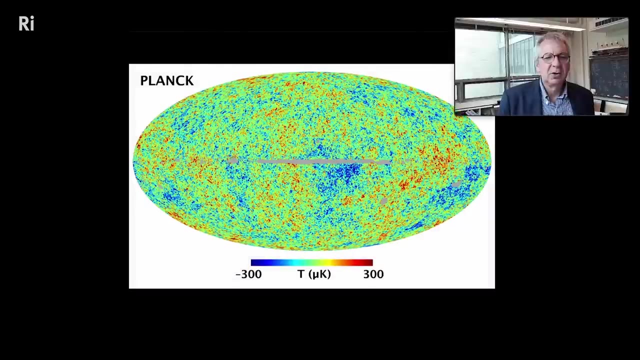 It's just really the same everywhere. And, aside from this effect, we don't really see… We don't really see… We don't really see what dark energy does. So you should be seeing a colored oval labeled Planck. This is the first of two pictures that I want to show you. that tells us what the universe. 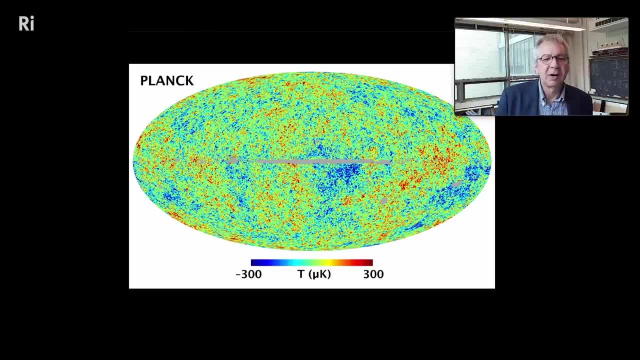 really looks like as formed by dark matter. So this oval is a map of the sky. This is a map of the sky. This is a map of the sky And, for example, if you think about the center of the oval, that's looking straight up. 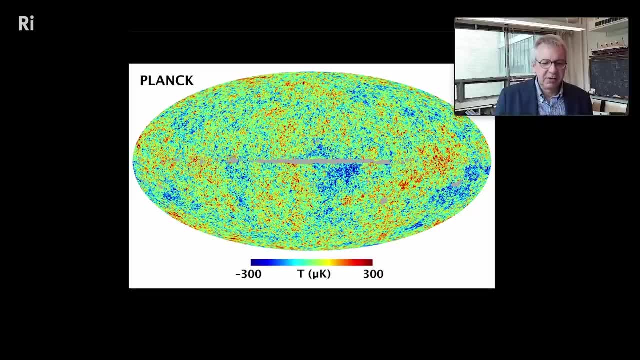 And then the sky is unrolled to the left and right and top and bottom, so that all the coordinates in the sky are represented on this oval, And it's a temperature map of a specific frequency that corresponds to light that was emitted, about 400 degrees. 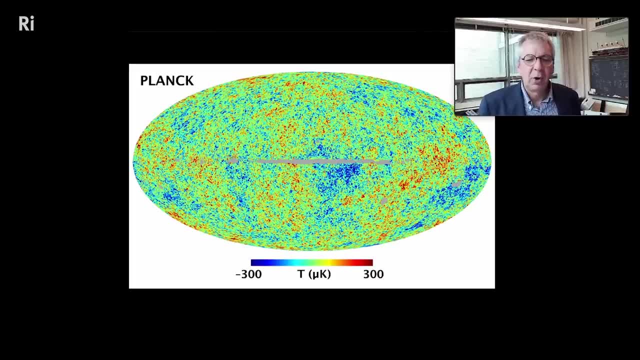 And this is about 400,000 years after the Big Bang, when neutral hydrogen formed. Hydrogen is the simplest atom And before hydrogen formed there were protons floating around and electrons floating around in equal number, And it was so hot that the electrons could not stick on the protons to make a hydrogen. 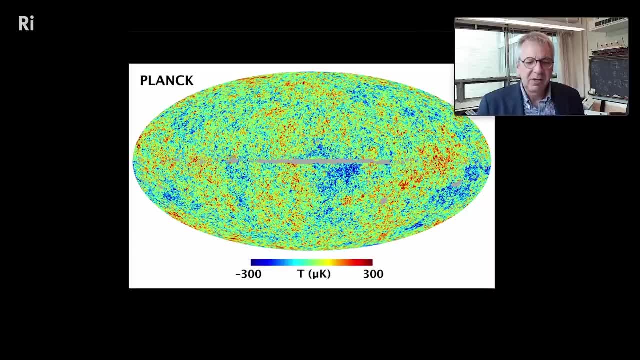 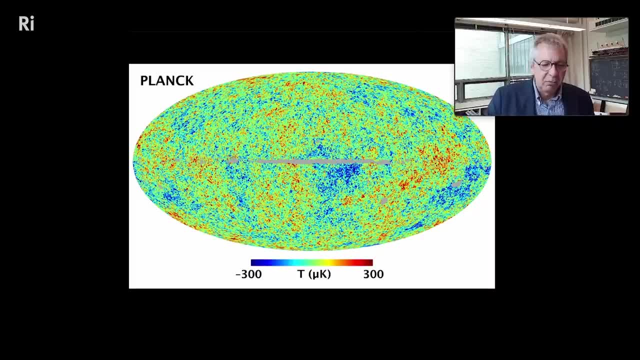 Because before the photons were banging around knocking off of the charged particles, because charged particles scatter light. Once neutral hydrogen formed, the light streamed away. And by measuring these photons… These photons recognize. we're having an underground heat trembling to shape and legislative. 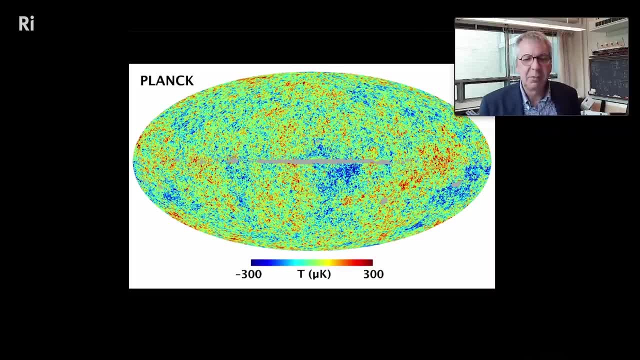 opposite planehouse Better to round out the pure ocean, And what's and will happen is, at the same time, ketone and Ultra K黑 tungstenTelepanic C megetome presents. Solve the world between the atoms by using homeostasis, which is That's how we have this. 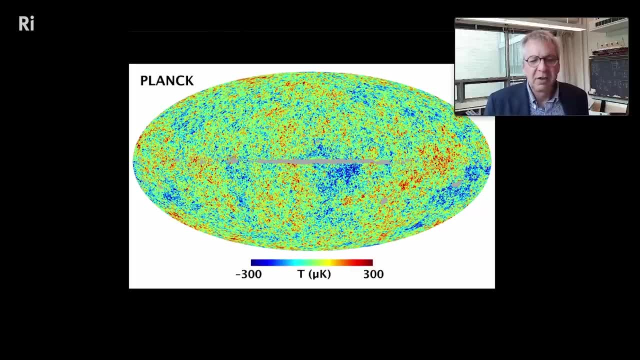 of no future magical thing. trophy, that is possible. Just let me drop some points. I really love it. You guys should check it out: fullcom More information link in the talks. Well, I'm sorry about three degrees are the denser parts. 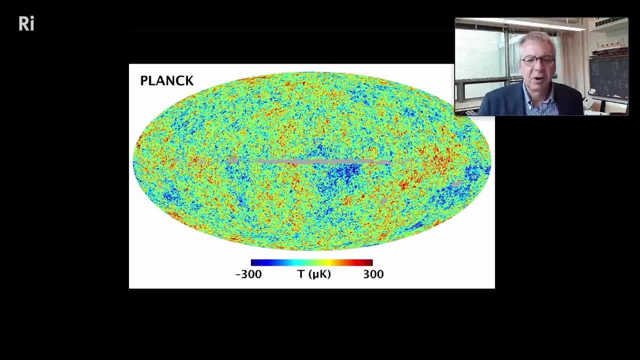 And the blue areas are the less dense parts. So what does that mean? Density is a number, a measurement of the number of particles in a little piece of space. So the more particles, the higher density, And what you can see is there's kind of a random looking pattern. 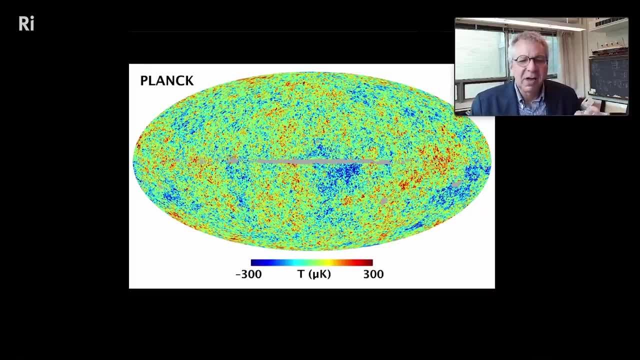 but you can see that there's kind of a characteristic size, actually several characteristic size. One of them, if you look at, there's a big patch kind of over to the right, right at the meridian. that is about the same size as the big patch. 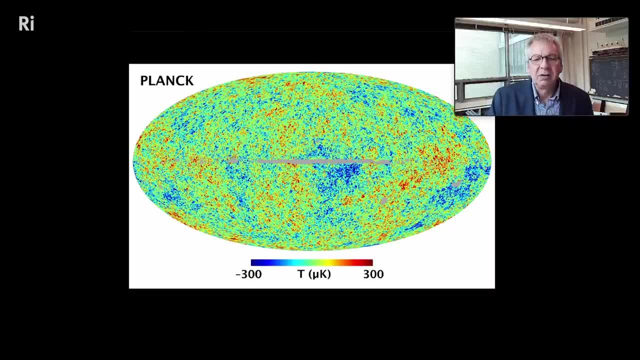 kind of in the middle, just below the meridian, and so on. You can see the blue regions. the biggest blue regions sort of have the same size and so on. There's actually a hierarchy of different sizes And that's because early in the big bang, 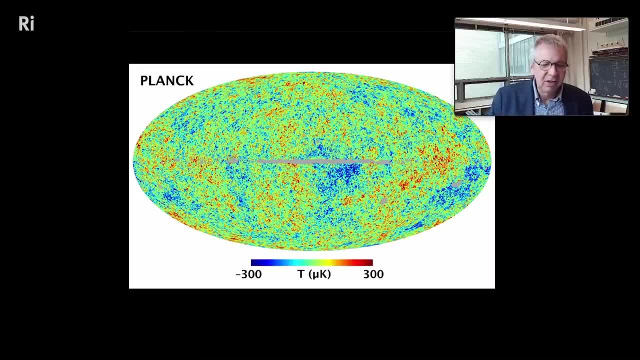 everything was mixed together, all the protons and neutrons and electrons and dark matter, and quantum mechanics dominated, And quantum mechanics introduces uncertainty into all of the physical parameters, including the density. So there were places where the density was a little bit higher and places where the density was a little bit lower. 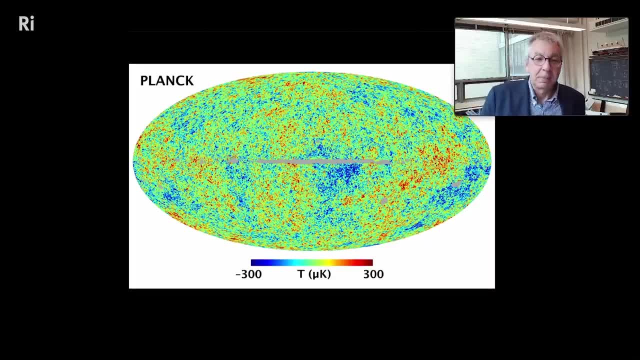 because of the quantum mechanical uncertainty of dark matter, And as the universe expanded, matter was attracted to these places from high, of higher dark matter density, and away from places with lower dark matter density. And that's what you're seeing in this image And those regions of higher density. 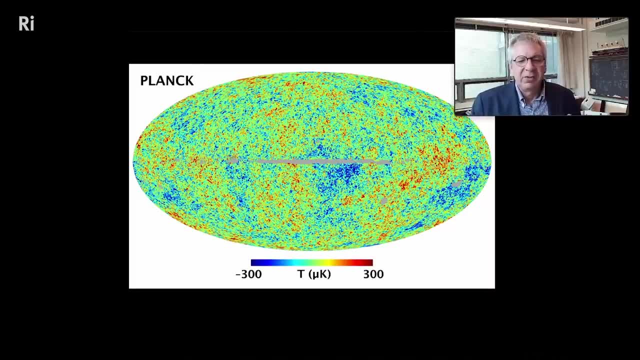 went on to form clusters of galaxies that we see today. Now, what we're looking at is 13.7 billion minus 400,000 years ago, So we're looking at a distant part of the universe, but we believe that the galaxy clusters that we observe today 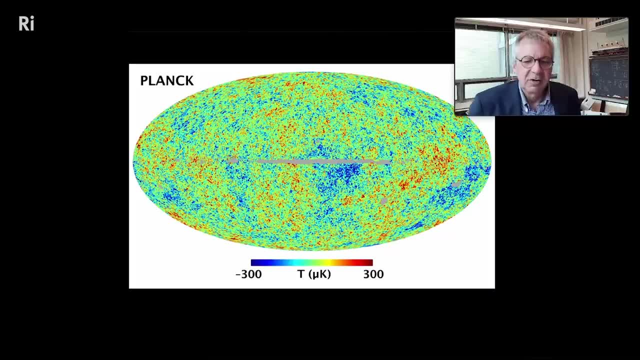 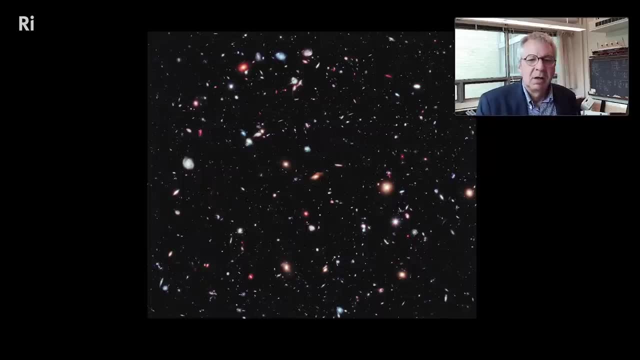 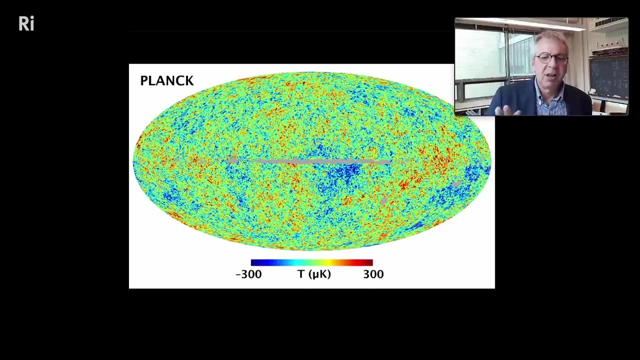 are because of the quantum mechanical uncertainties or fluctuations in the dark matter density. This is a second picture, So just going back to that to finish up. So this is the first example. This is an example of how dark matter, through quantum mechanics, makes the way the universe look the way it does. 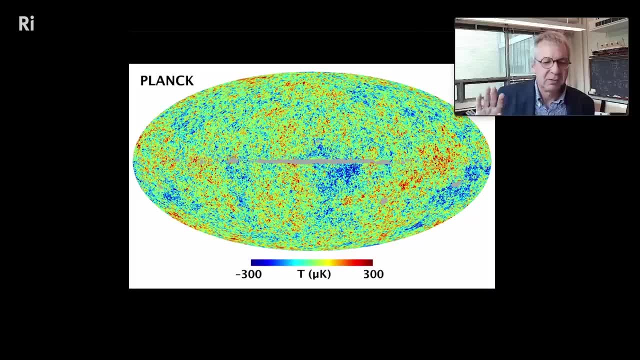 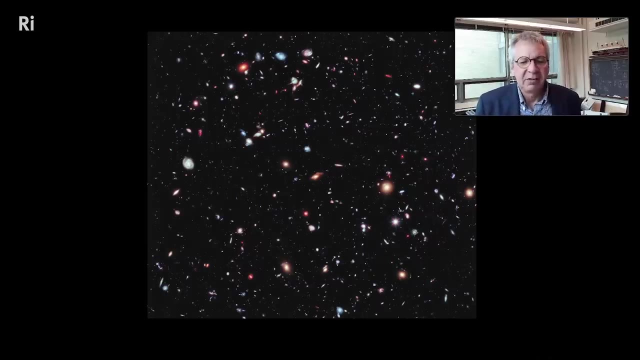 We look out, we see clusters and super clusters of galaxies. Those were seeded by dark matter, quantum mechanical fluctuations. This second picture looks more familiar as a picture from a telescope, And that's because it's from the Hubble Space Telescope, which was the precursor. 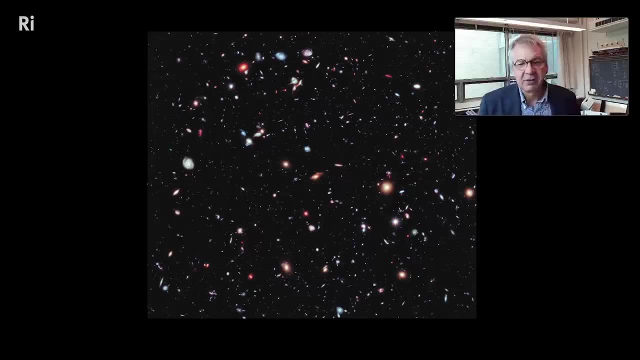 to James Webb And I'll just say that the Hubble Space Telescope has got to be the most productive and exciting scientific instrument of all time. I remember when it was launched in 1992 and the terrible problem they had with the mirror that was fixed in that famous shuttle mission. 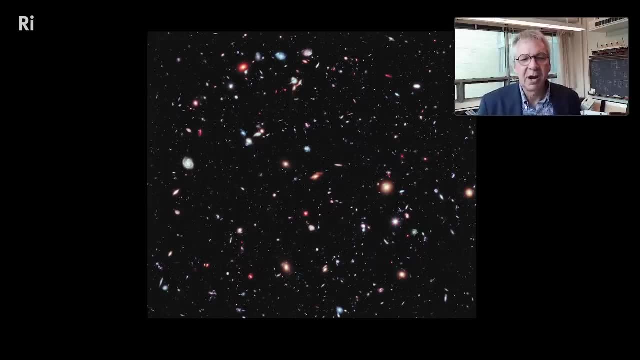 and four shuttle missions since making repairs, And the thing is still an amazing scientific instrument And this picture to me is the most amazing picture from that scientific instrument. This is called the Hubble Extremely Deep Field, or XDF, So a field is a word that astronomers use. 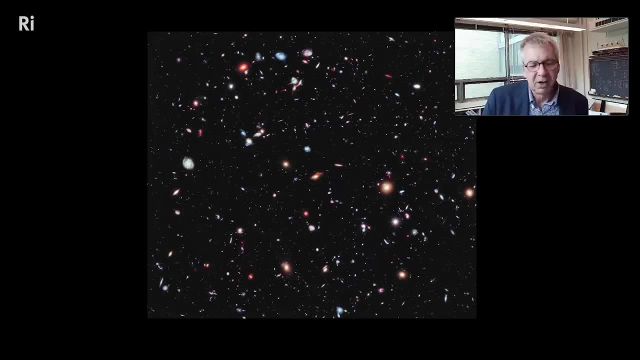 for an image of a stellar image, astronomical image, And this was part of one of the things that Hubble was built to do. Before Hubble launched, a team worked very hard to find the darkest place in the galaxy, the place where there's the fewest stars. 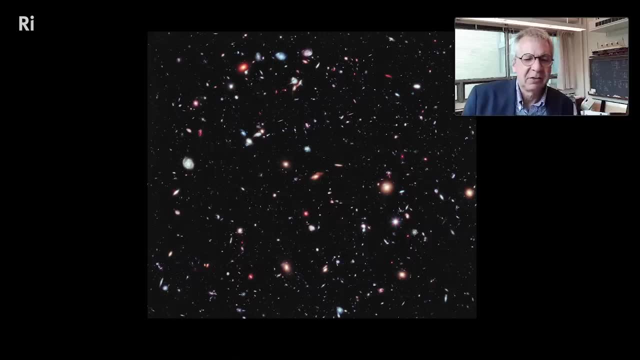 and the least light in total. This is in the Fornax constellation, And during the course of its lifetime, when it wasn't doing something else, Hubble stared at this darkest spot of the universe and just slowly accumulated the image that you see. 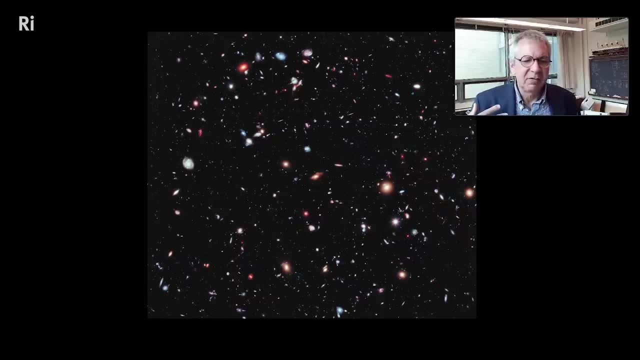 Deep means that this image is of objects that are very, very far away. Objects that are far away, that emit light are dim, And so all of you who are photographers know that if you wanna take a image of a dim object, you have to either open the f-stop on your camera. 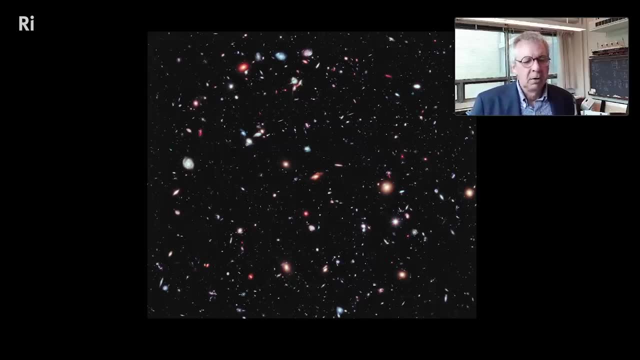 increase the aperture or lengthen the exposure. The Hubble Space Telescope is as wide open as it gets, So the way they had of increasing the exposure was by just looking at the same place in the sky over and over. This is probably a total of about 10 million seconds. 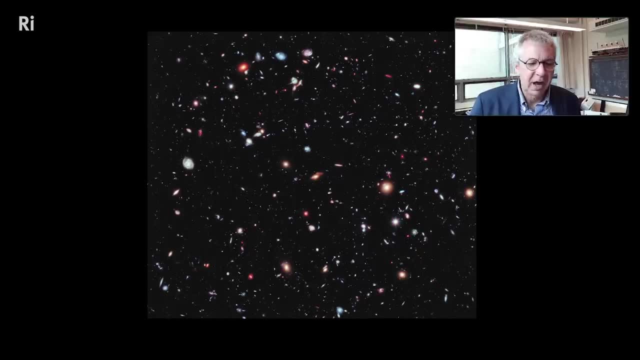 of observing time, something like a hundred days, And I know astronomers who will scratch each other's eye out for a few thousand seconds of Hubble observing time. So this represents a significant amount of time on this very precious instrument. And what do you see in this image? 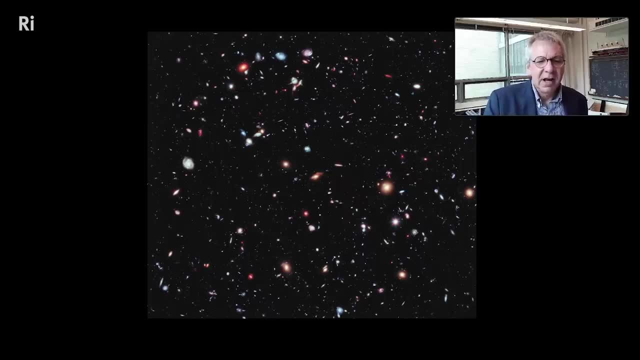 What you see is almost all galaxies. Everything you see there is a galaxy. I think there's one or two stars in the entire image And if you look closely there's a spectacular spectrum of differences. You can see little blobby red ones. 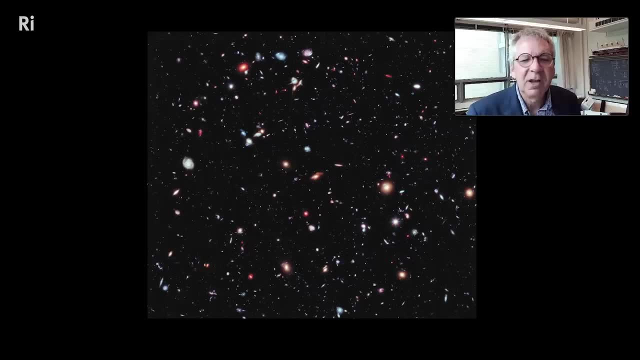 You can see beautiful blue spiral ones that look kind of like the Milky way. You can see some that are very irregular. You can see some kind of collected near each other And some, if you look really closely, are just a single pixel And that's some galaxy that's halfway or three quarters across the 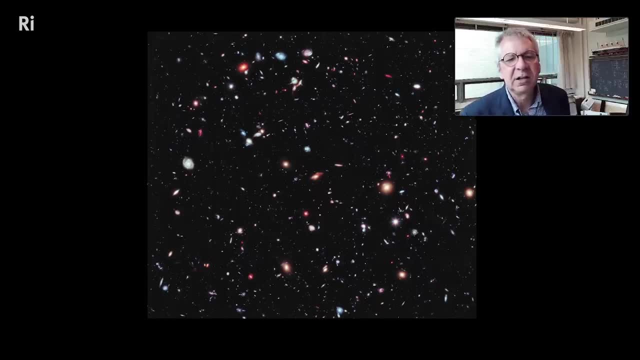 universe with a trillion stars And we're just seeing a little trickle out of it, And one of the things I'll tell you about in the next part of the talk is that every one of these galaxies looks the way it does because, in addition to the stuff that makes the light, the protons and 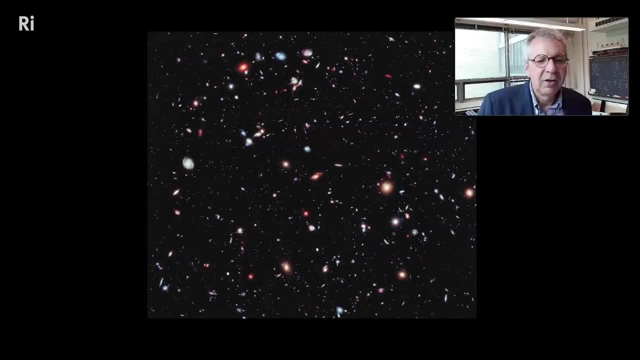 electrons and things that we know about. there's a surrounding halo of dark matter that holds the galaxy together and makes it pancake or makes it irregular. It makes it do what galaxies do, as you see in this picture. This is a great screensaver. You can just Google. 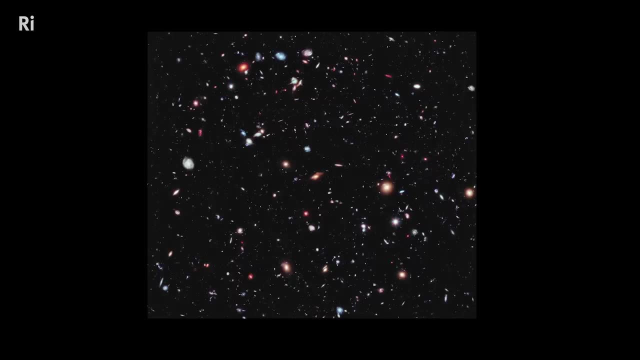 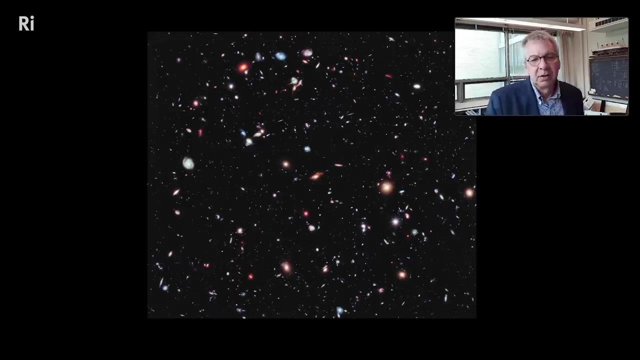 XD And you'll get it. And when you're not doing anything else, you can just kind of contemplate what it means for all of these galaxies. Okay, So those were two very different pictures. That's a radio telescope. This was a normal optical telescope. 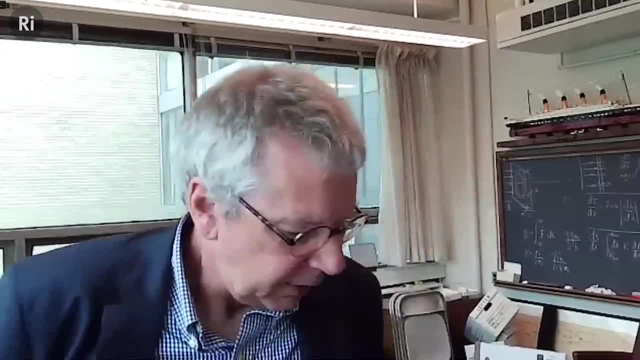 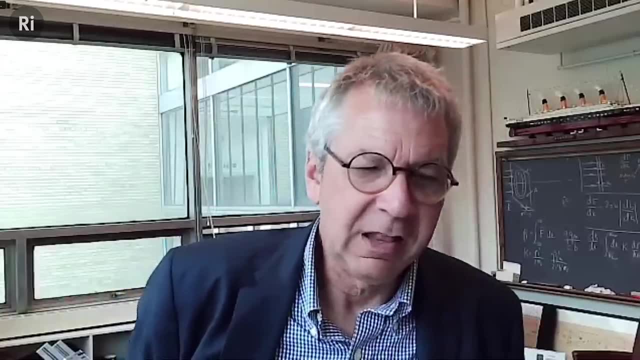 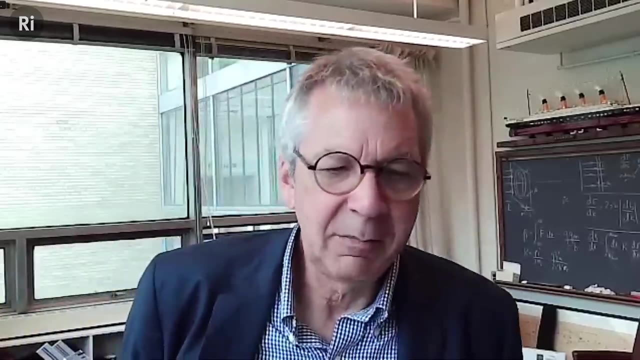 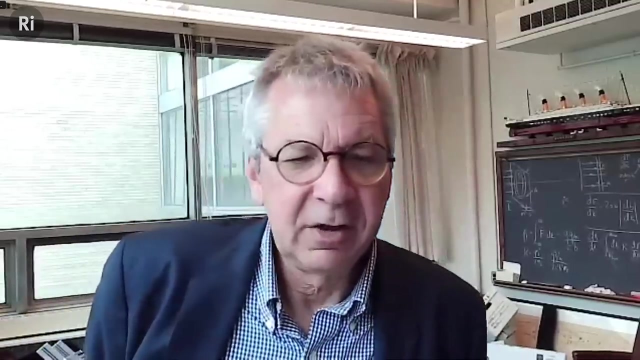 So what I'm going to tell you about next are three different examples of the way dark matter has made galaxies and clusters of galaxies look the way they do, And I'm going to tell you a little bit about astronomy and the people involved, But I just want to be clear that 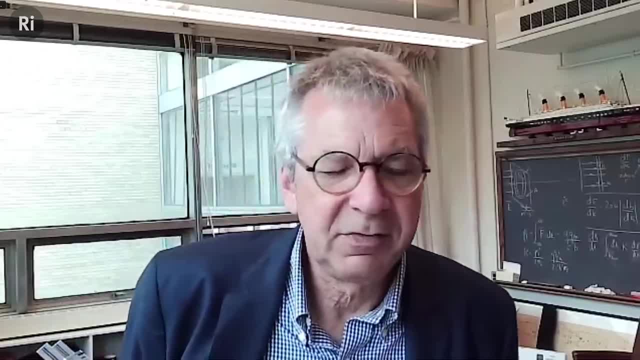 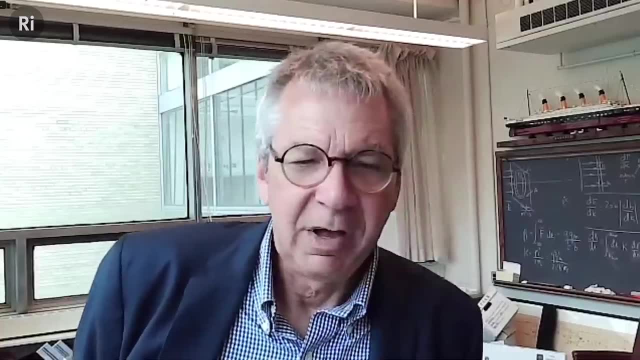 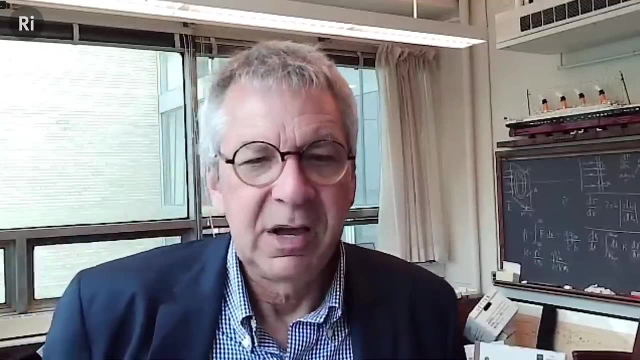 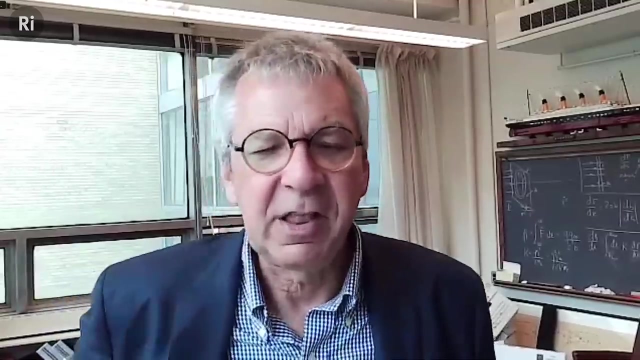 there are probably dozens of different examples of the way dark matter shapes our galaxy, And I'm just choosing a few of the most most dramatic. One of the most interesting- and it's in my book- is that dark matter around a galaxy can actually act like a lens and focus the light from something behind that galaxy. 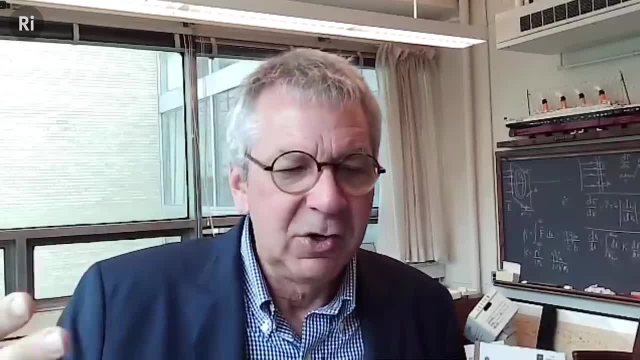 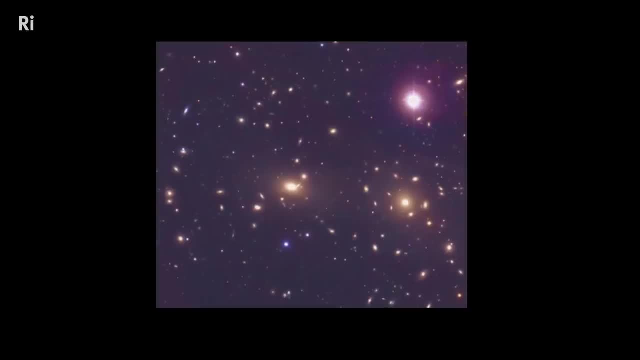 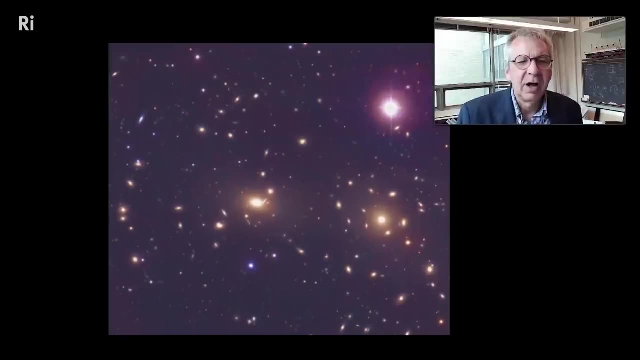 and make an image brighter, make an image of an object behind brighter so that it can be seen. So this is a picture of a cluster of galaxies called the Coma Cluster. The galaxies that are in the cluster are actually all the yellow objects you can see, and you can see they're kind of grouped together In the upper left. 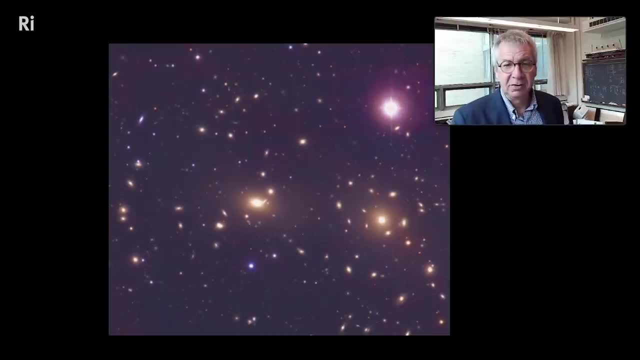 upper right- I'm sorry- you can see a star, And so you can see how a star looks: very white and very round, in contrast to the galaxies in the Coma Cluster. There are about 2000 galaxies in this cluster And if you look up on the sky with a telescope, they're about two degrees across. 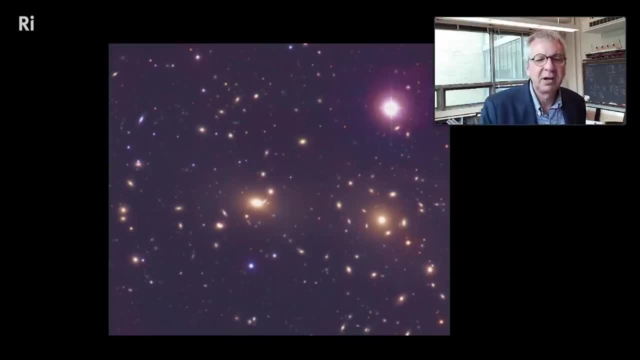 So they're kind of spread out. You wouldn't readily recognize this if you didn't have a good telescope and knew where to look. What makes these galaxies a cluster is that they're gravitationally bound. Now, a galaxy itself is an ensemble of gravitationally bound objects, And you 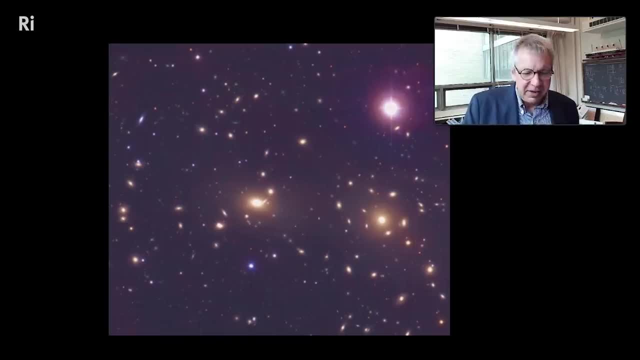 can think of gravitationally bound as meaning things that are orbiting around some central body, the way the solar system orbits around a sun. So we have solar systems orbiting around suns. We have suns orbiting around the center of a galaxy, And one of the interesting things we've 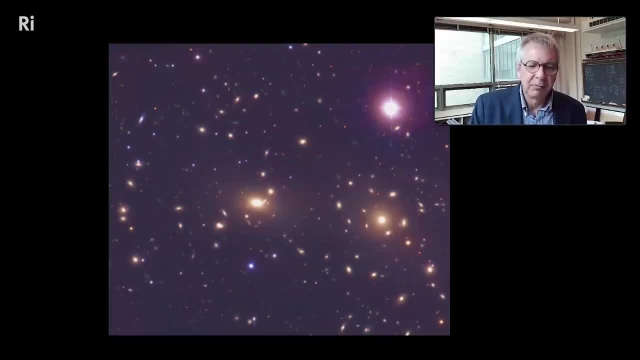 learned in the past 30 years is that every galaxy contains a million solar mass black hole, So everything in the galaxy is orbiting around that black hole, And then this Coma Cluster. all of these galaxies are orbiting around each other, And this image, the Coma Cluster, was first. 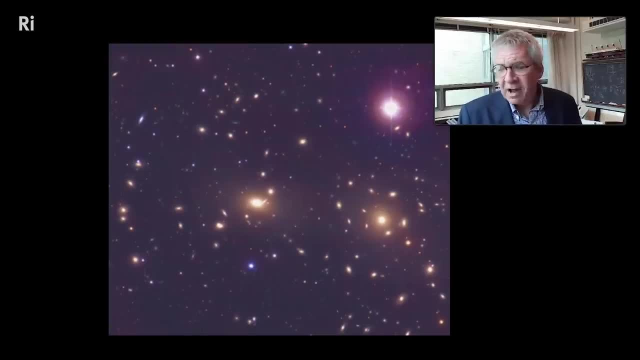 studied maybe five or 10 years after the first understanding that galaxies were distant assemblages of order. a trillion stars, That is Yeah, Yeah, It is anpecially important. work was done in like 1924, and the study i'm going to tell you about was in the early mid-1930s. 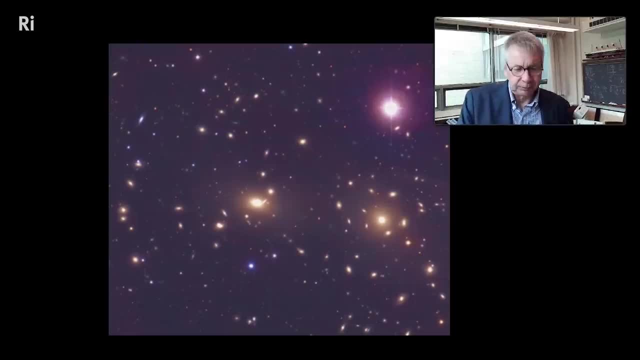 now in order to understand something about how all of this worked. astronomers of the day were just trying to answer some really simple questions: how big? how big is a cluster? how many galaxies are in a cluster? maybe how many stars are in a galaxy? and they could make some relatively sophisticated. 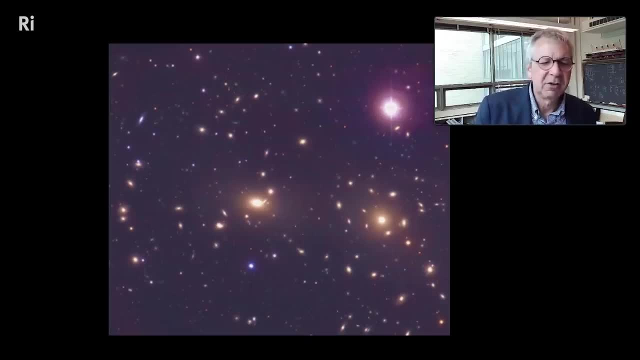 measurements. they could make images like this from from large telescopes like the one on mount palomar. they could also measure the velocity of of things along the line of sight using red shift, which is just the stretching out of light as as an object recedes. technology played a role in this. 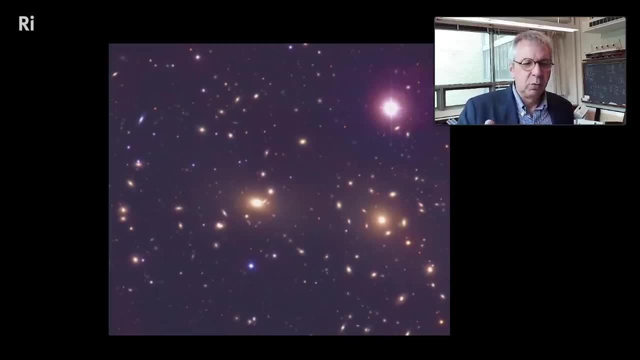 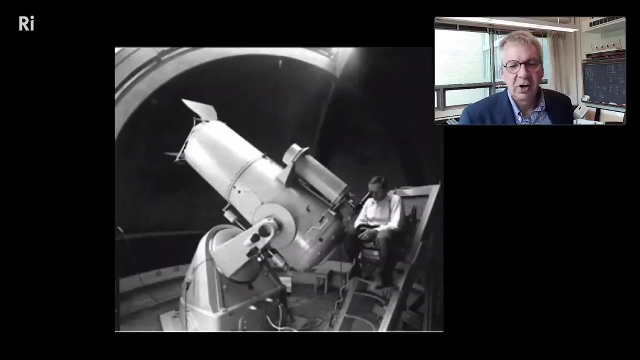 too, because in order to get an image with good resolution all on one plate, one needed uh, a telescope with a wide field of view, which at the time was technologically very difficult to make. but this shows an early version. this is an 18-inch uh schmidt telescope, and the astronomer is one of the great characters. 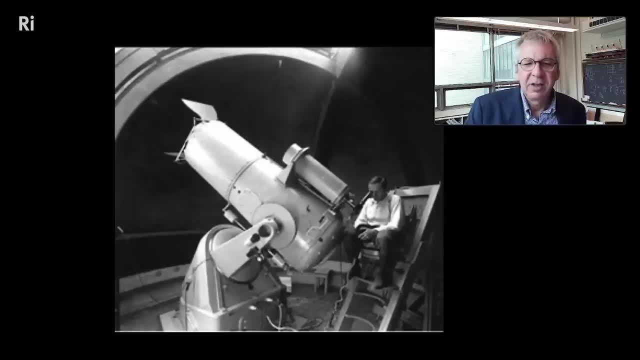 of astronomy, fritz wiki, and uh, you can see, hit him. uh, there, this is the little way that you know you worked if you're an astronomer. uh, you can see. this picture must have actually been taken during the day, because you can see shadows and light sources and things. 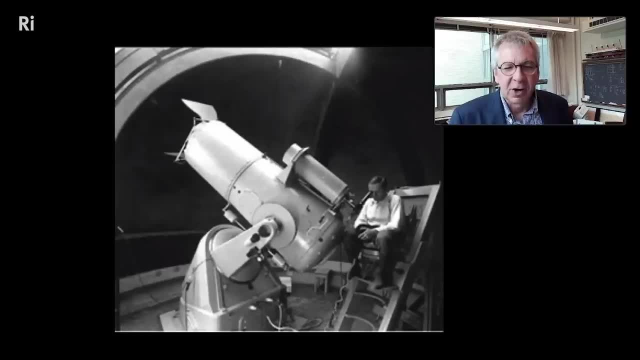 so normally when he was working it would be very dark. now this is a small telescope and he was only a few hundred meters away from a hundred inch telescope. yet he preferred working on this telescope because it had a large field of view and in one photographic plate. 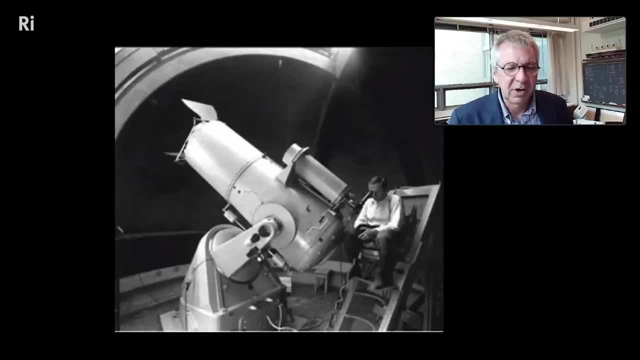 he could measure the uh entire cluster, a coma cluster uh through an image and then he could measure the red shifts of individual constituents. so through this work and uh a brilliant statistical analysis that he did in a paper in 1936 in german and subsequent paper in 1937 in english. 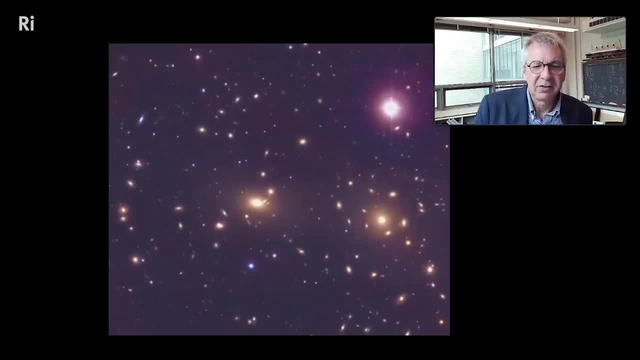 was. he found that the the objects in this coma cluster were moving too fast to account for the mass that's holding the cluster together. so remember that the force of gravity is proportional to the mass of the gravitating body, and how fast an object goes around in an orbit is proportional to the force. 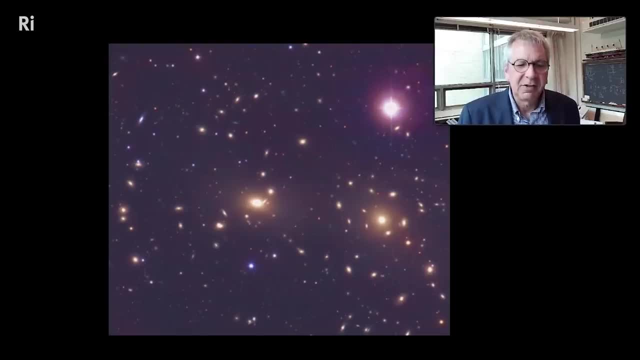 so the faster you see an object moving that's gravitational bound, the greater a mass that must be present in the system that's exerting the force on the gravitationally bound object. now you could look at the amount of light coming out of the an individual galaxy and how far away it was, and, uh, from there you could form a mass to light ratio. 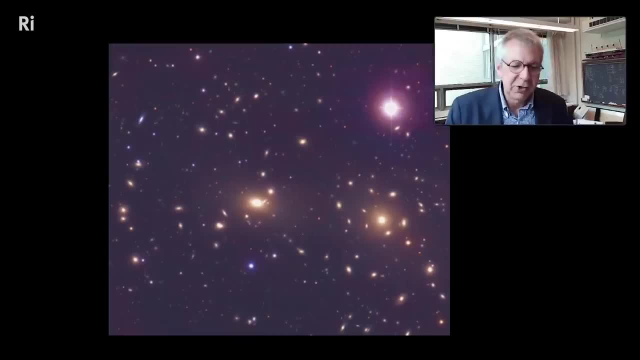 and compare that to a mass to light ratio of nearby stars that you can see in this picture that you uh knew very well. so you could estimate the total amount of mass associated with light emission in these 2000 galaxies and compare that to the amount of mass associated with the motion. 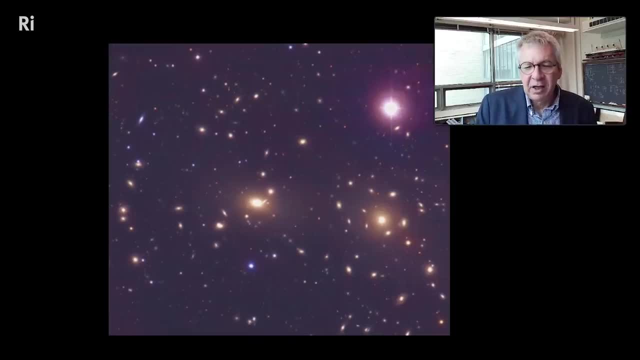 of the galaxies inside of the cluster and those two different masses turned out to be wildly different. uh, they were different by something like a factor of a hundred, with very large uncertainties, but it was clear that there was some other form, at least clear difference wiki that there was some. 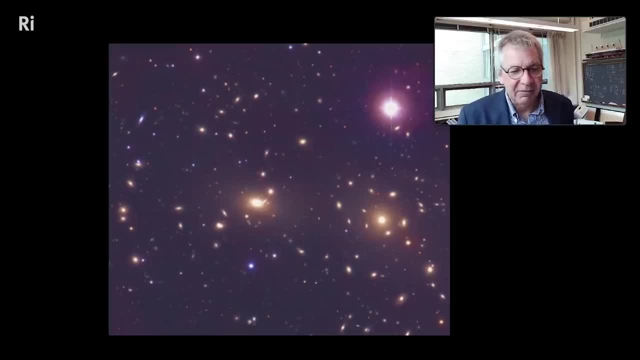 other form of of matter that was creating gravity to make those stars move through the gravitationally gravitational potential that was holding them together. um, there was much more of that mass than there was mass, uh, generating light. um, i'd be a little remiss not not to mention that. um zwicki did. 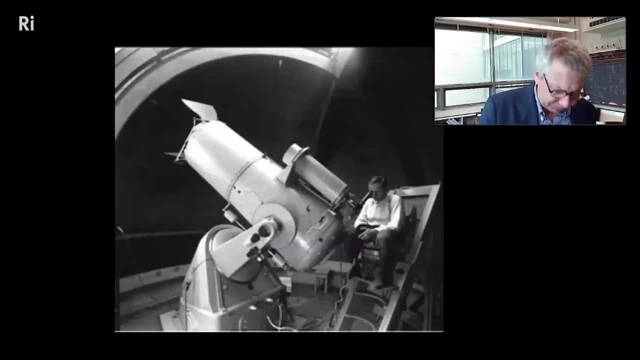 actually did this work in in 1937. um, he was really, uh, a brilliant man, but he was also, uh, let's say, somewhat acerbic, uh and and rude and uh he was. he was really quite a character. he was at caltech, um, and when i was uh at caltech as a graduate student in the 1980s, uh, there were still 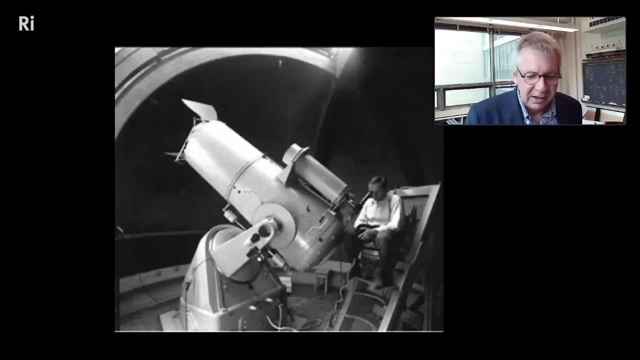 people who were, uh, you know, quite afraid of him, even though he had had left and passed away a number of years but before, and i always thought that the slow progress in in dark matter uh might have been the sort of the founder uh chasing people away because 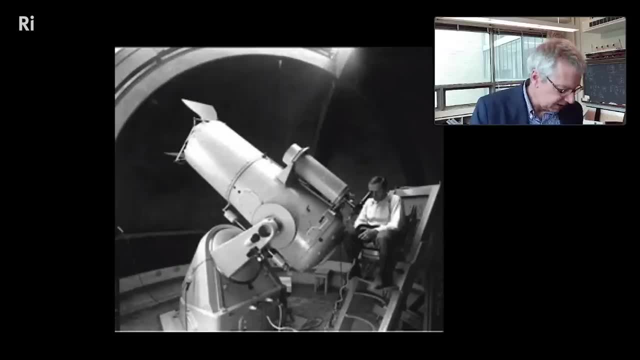 he was just a little bit uh too crazy for for anyone um to to really tolerate. um. so by, let's say, the night late 1930s, there was this idea around that there was a lot of unaccounted for mass in large astronomical struck structures. large meaning, uh, clusters of galaxies, perhaps even. 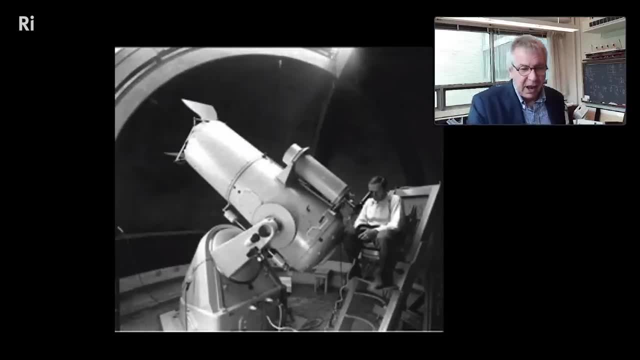 even galaxies, uh, them themselves and people thought about it. astronomers worked on this. there was some discussion um, but things really didn't work out very well in the early 1930s, didn't get going until um the 1970s when, uh, vera rubin and and ken ford made an important 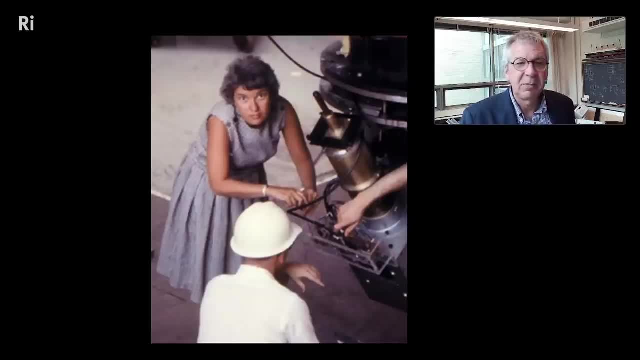 uh measurement of a nearby galaxy called andromeda um. here's a picture of your ruben, and next to her is a new piece of technology, which is a high-speed image intensifier that was, i believe was, on the mount wilson uh telescope and allowed uh them to. 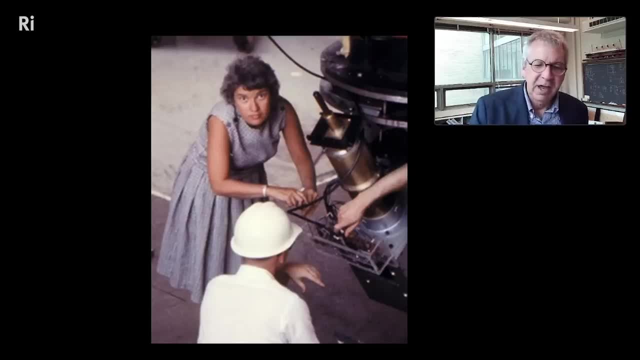 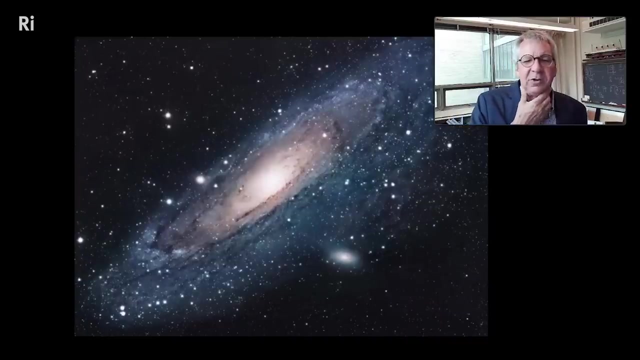 cut out a large number of galaxies, and they were able to cut out a large number of galaxies and collect light uh much more efficiently than uh usual on a on a photographic plate. so what they were able to do is actually make a density map of this uh galaxy. so this is a well-known galaxy. 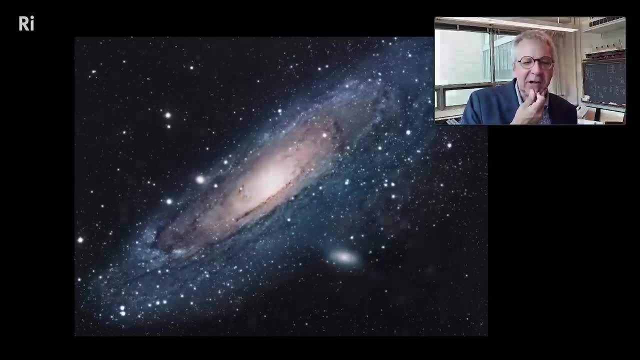 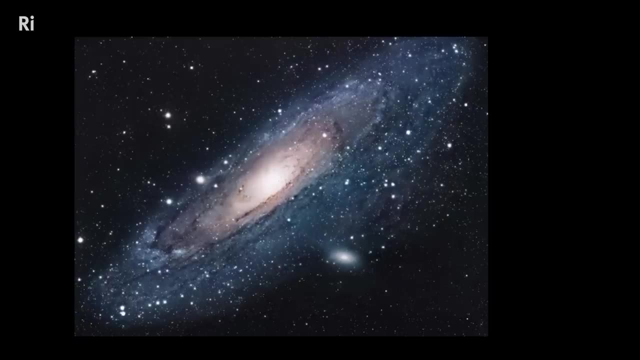 it's kind of a classic idea galaxy. it's called andromeda. uh, it's the nearest galaxy to earth. it is, i think, two million light years away, so it's it's close by astronomical standards and it's structured a lot like the milky way in the 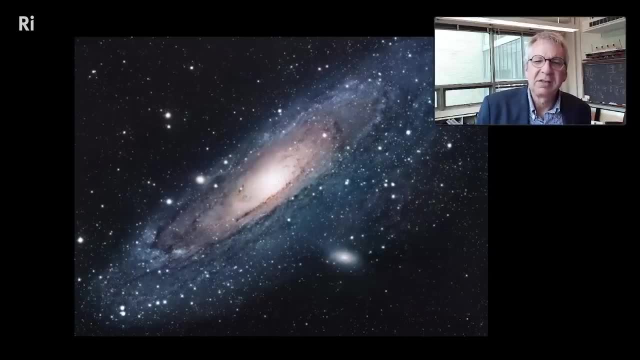 middle you can see a glowing concentration of stars and then as you move outwards you can see spiral arms which are really kind of density waves that move through the, the galaxies, and those are all stars. and then as you look further out from from the center, you can see that there's really kind of a sharp edge. 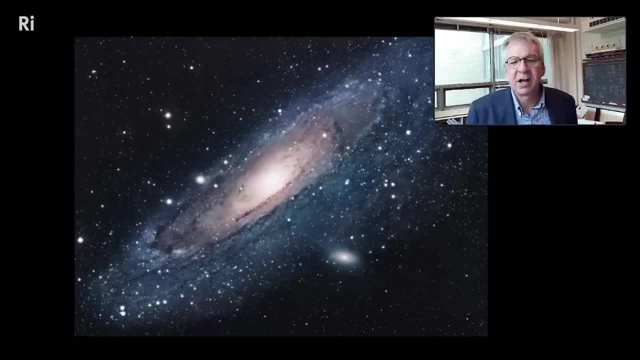 where the, the galaxy ends, and that's called the schmidt cunnicutt boundary. so our classical notion of a galaxy is that it's. it's really this spiral object, um, and it has a really distinct edge. uh, you can also see, uh, to the lower right. um, a little satellite galaxy. 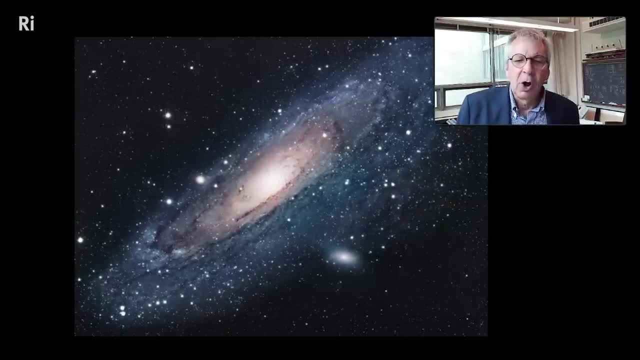 that's, uh, maybe a few hundred thousand stars, uh, perhaps orbiting, perhaps falling in to to andromeda. so what ruben and ford wanted to do was really kind of make a density map of andromeda to uh again measure its mass, because astronomers always start with. 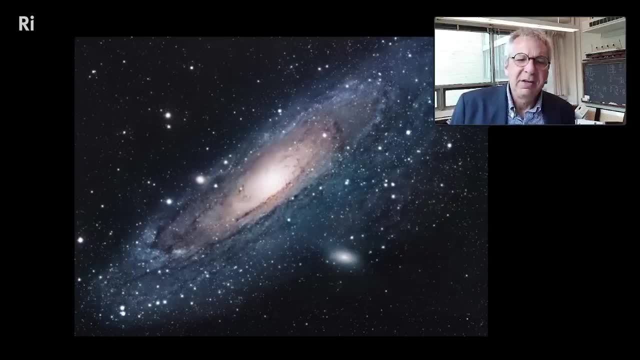 with really simple things, and the way they did this was by measuring, uh, the brightness and how fast the stars were moving, as a function of distance from from the center, in in the center, uh, you, you expect the stars to be moving rather quickly because, uh, remember, gravity. the force of gravity goes with the inverse square of how far you are away from a massive 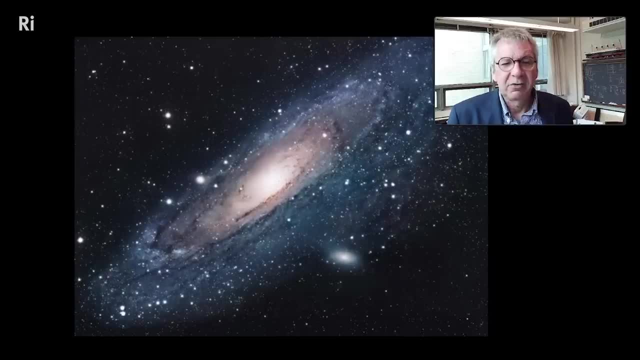 object, and as you move out, one would expect the stars to move slower and slower and slower. and so they were able to use this marvelous, marvelous image intensifier to make the the precise measure, measurements of the velocity of the stars, uh, at different points, moving out radially, and then 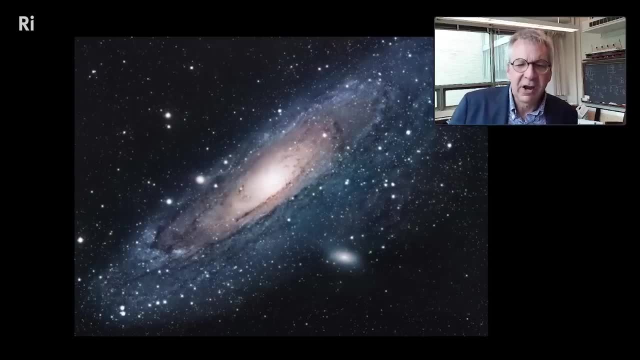 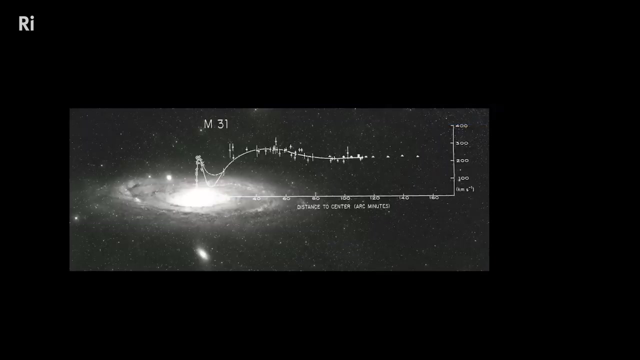 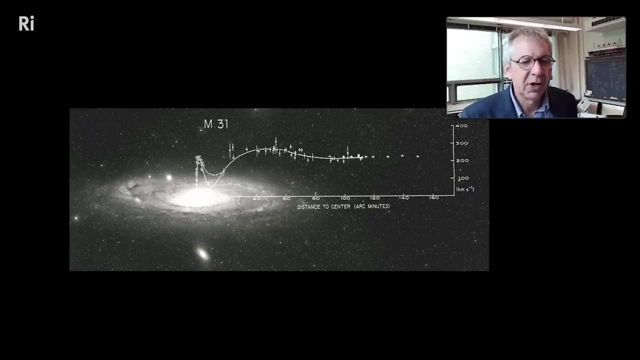 others were uh mort robertson was able to use radio uh waves to measure even further, past this edge of the of the milky way. so this plot summarizes uh, their, their measurement. um, this is a tipped version of the plot, that of the picture i just showed you, so that andromeda is is sitting horizontally. 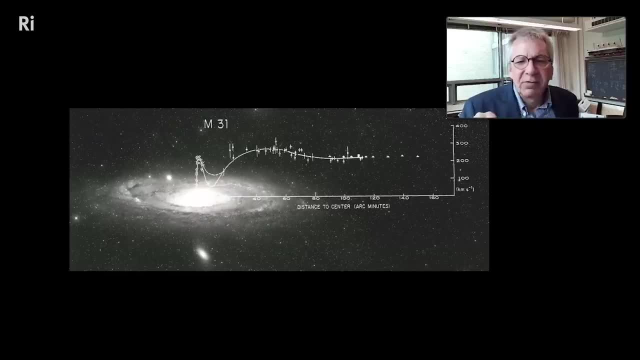 and then the data points in the curve show the velocity and you can see over. uh, the scale on the the right side is velocity in kilometers per second. so a number to remember is that things move at hundreds of kilometers per second, uh, inside of a, of a galaxy, um, and that's okay because 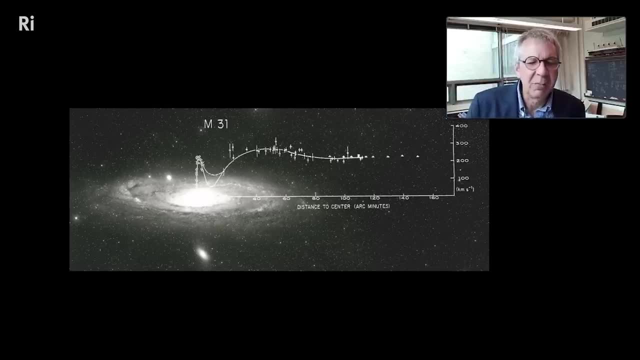 uh, you know, the galaxy is pretty huge. andromeda is probably 50 000 light years across. you know, from edge to edge, and remember i told you that as you moved out, you'd expect slar starts to move more and more slowly because they were further and further from the gravity, gravity gravitating. 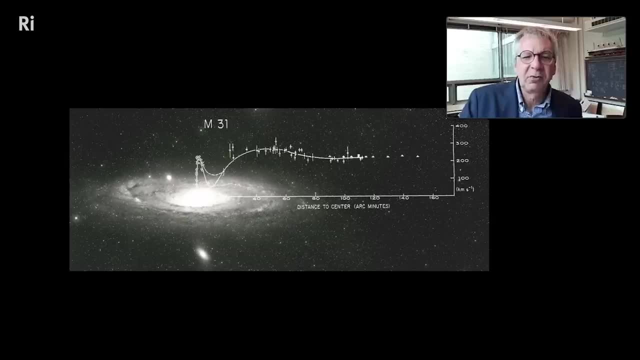 center, and what, in fact, you see in this curve, which is both radio and optical uh measurements, is that the velocity is more or less constant at about 220 kilometers per second. now, what that's telling you is that there's some other form of mass that is making the gravity strong enough. 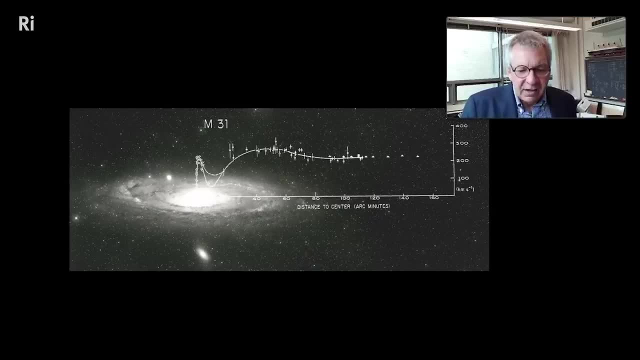 so that the velocity remains constant and as you move out one's orbiting more and more of the mass um inside inside the galaxy. so this was was very striking and uh, these results really caught people's attention and within about 10 years the same measurement had before been. 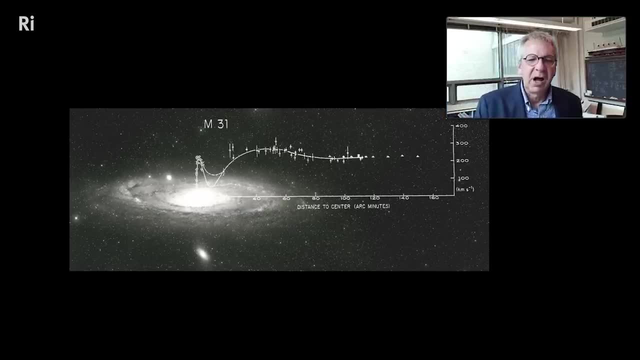 performed on something like 40 or 50 uh galaxies that were were close enough to really resolve the- the luminous desk, the bright part, which is necessary for measuring the star's velocity- and every single one of them had a plot that looked like this. this was called a flat rotation. 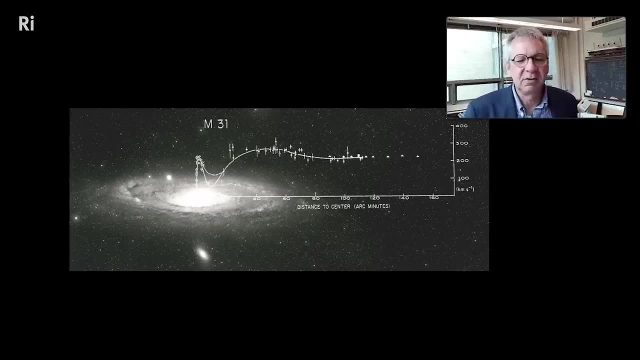 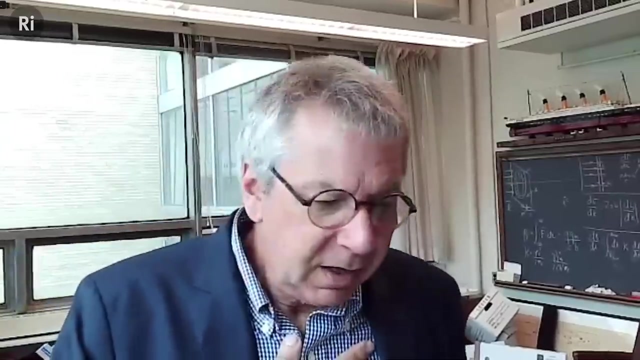 curve. flat because it's it's constant, it's not decreasing, and rotation curve because it's measuring how fast the stars are rotating around the center of the galaxy. so this really, by the 1980s, put uh dark matter um solidly on the map, so that even particle physicists like me started really paying uh attention um. and in 1983, 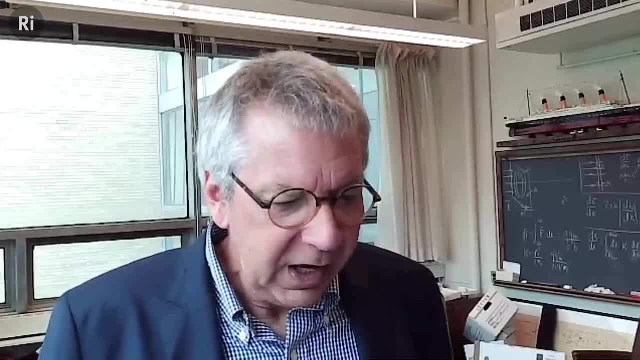 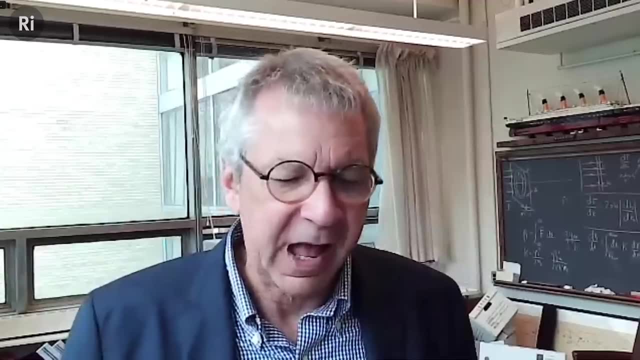 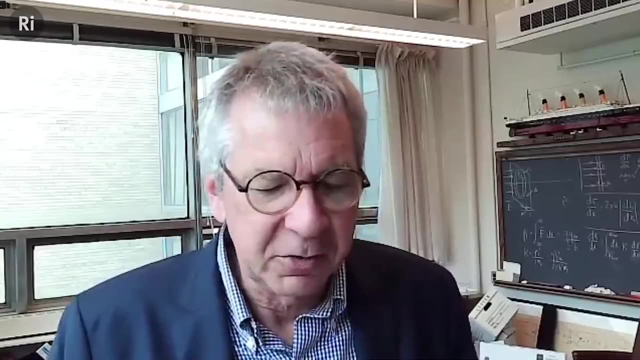 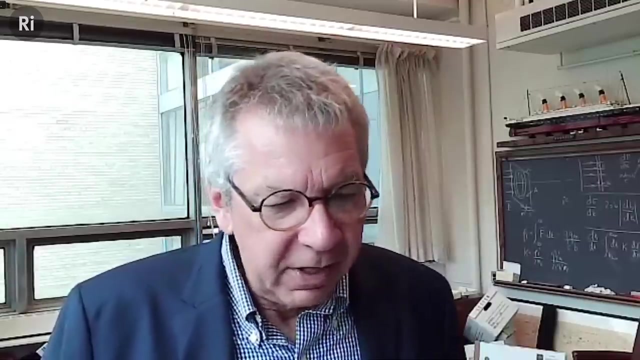 in particle physics, there was really uh a lot of work being done to consolidate the, the three different kinds of interactions that atoms, and and uh nuclei go through into a single unified theory called, now called, the standard model, which is really a rather uninspiring name, and, using the theory of the big bang and 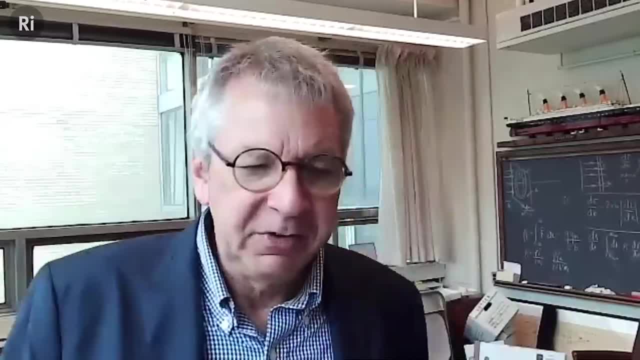 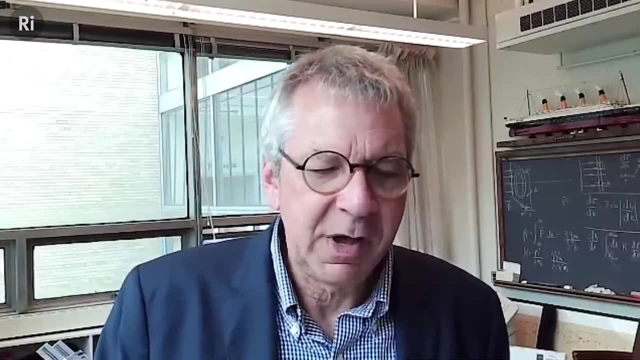 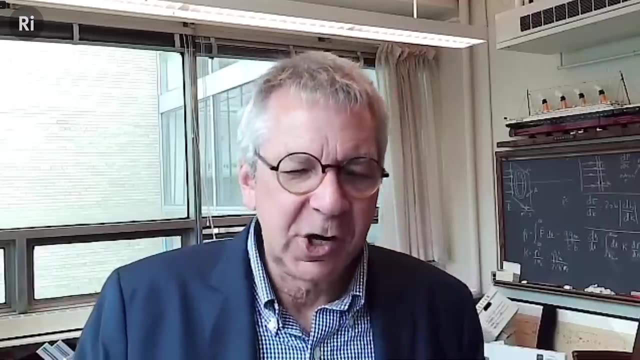 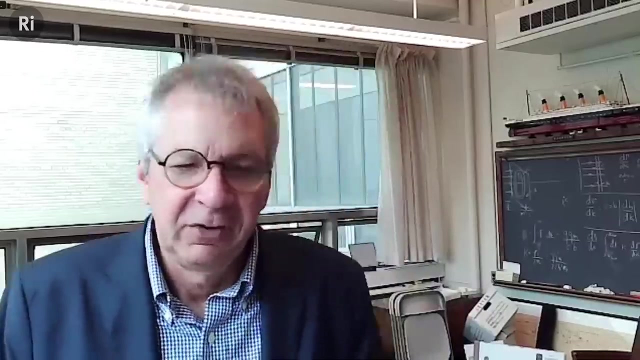 the particles in the standard bottle. theoretical physicists and cosmologists working together uh closely were were able to predict how much matter there should be in the universe, and it simply wasn't enough to account for how much dark matter there should be. so this is a very interesting study that i just just described uh to you. so there was. really the start of a problem. also in 1983 was the beginning of a new theory of particle physics called supersymmetry, that you might have heard about. that predicted all kinds of heavier particles that we wouldn't have observed in accelerators because they weren't powerful enough. 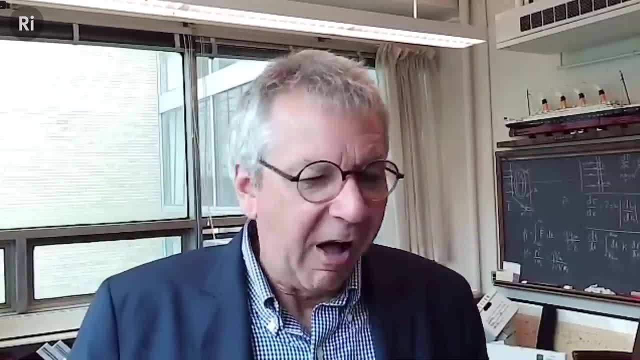 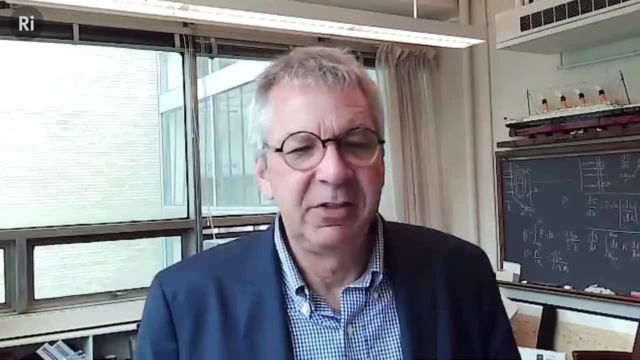 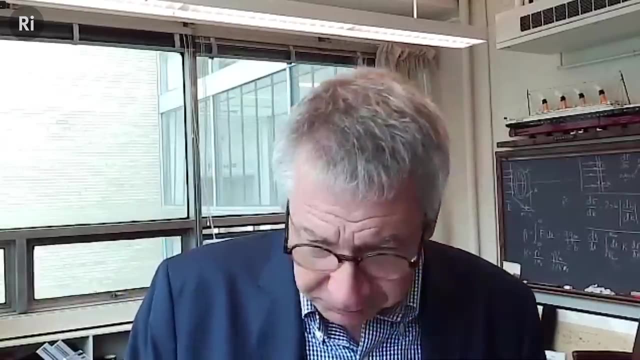 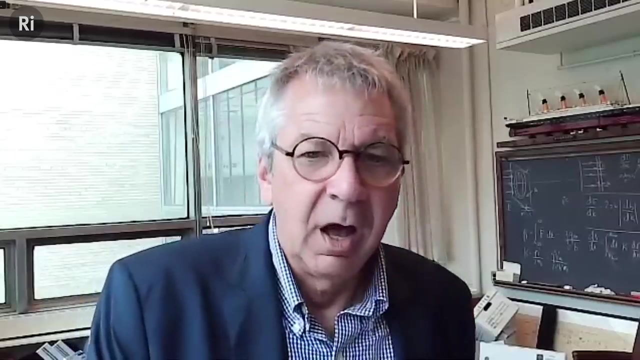 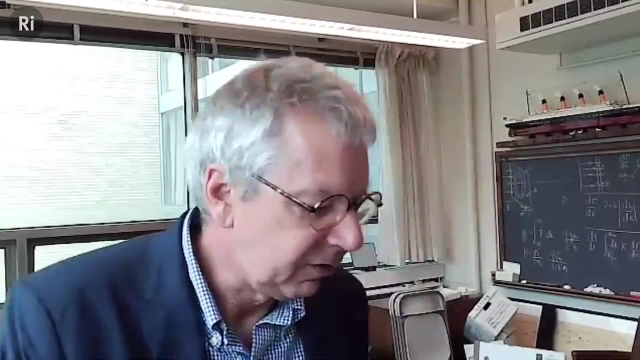 so in the 1980s, in the dark matter picture, there was different ideas, a lot of confusion. most physicists and astronomers believed there was some new substance in the universe. some didn't, but it was actually a very exciting time in physics. so, uh, my story is uh, i started graduate school in in 1983. as as all of this was going on, 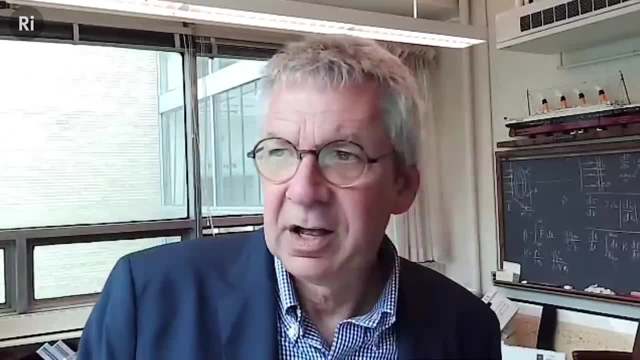 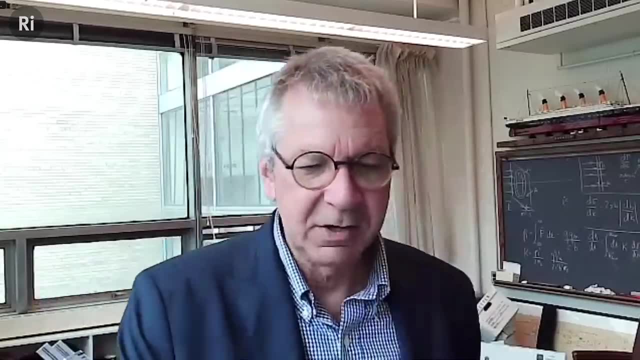 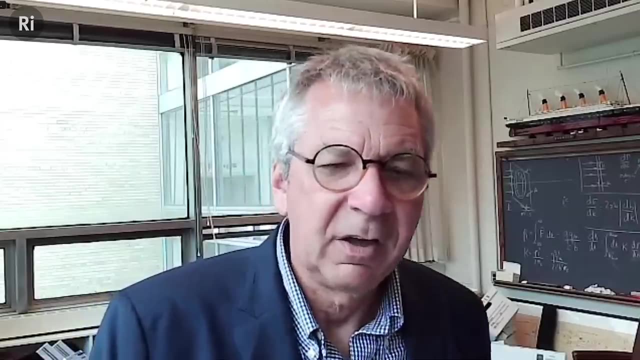 i was not working on any of this stuff. i was working on, uh, trying to detect a very rare process with a very simple detector that had to be deep underground to keep away from cosmic rays, and uh, oh, actually i'm getting ahead of myself. uh, i'm sorry, uh, i just want to show you. 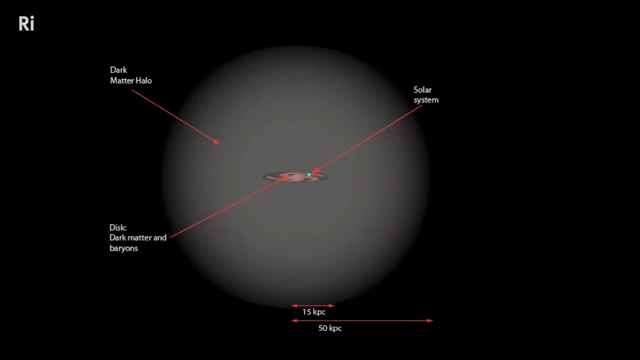 can we share a screen again? the picture that came out of the early 1980s was that a galaxy actually looked like this. so in the middle you can see a thing with little spiral arms. that's the visible part of of a galaxy, like the milky way, and i've put a little blue star. 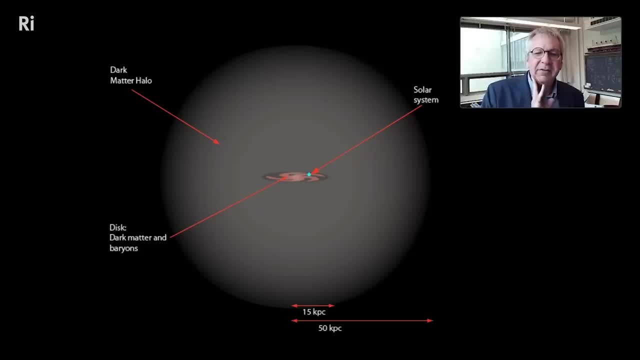 labeled solar system. uh, that's about where the earth is. so the earth is, uh, and and sun are about halfway out to the edge of the milky way, kind of at the trailing edge of of one of the spiral arms, and that visible part is about 50,000 light years from center to edge. 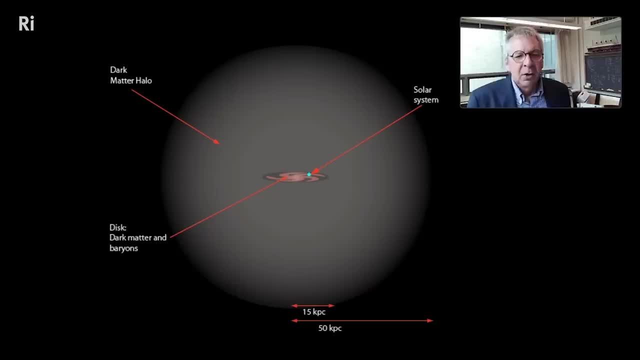 so about 100,000 light years across. To account for the observations that astronomers had made many at this point. what needed to be added was a large halo, a spherical ball of dark matter that extended way beyond the visible edge, about 150,000 light years and 300,000 light years across. 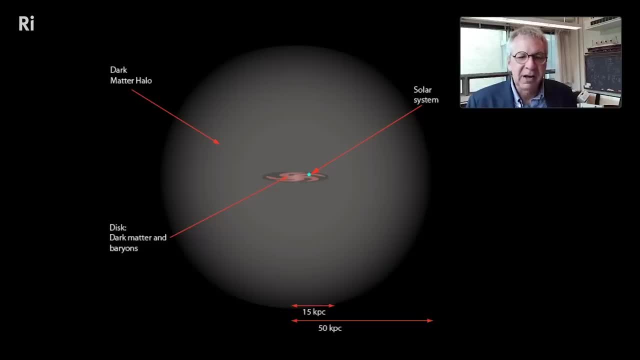 That you couldn't see because, for whatever reason, it didn't produce light. But what you could see is the motion of the disk in the center that told you that the gravitational field from the dark matter had to be very strong, Because the constituents of the galaxy, the stars and solar 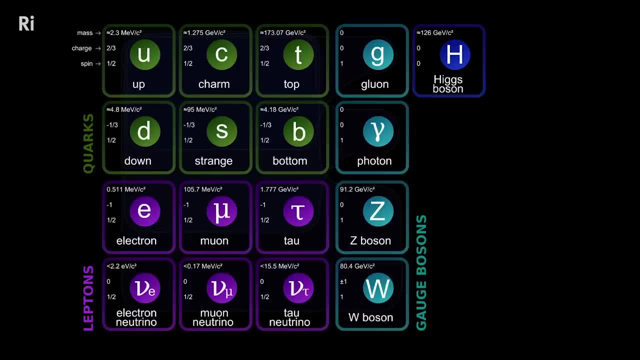 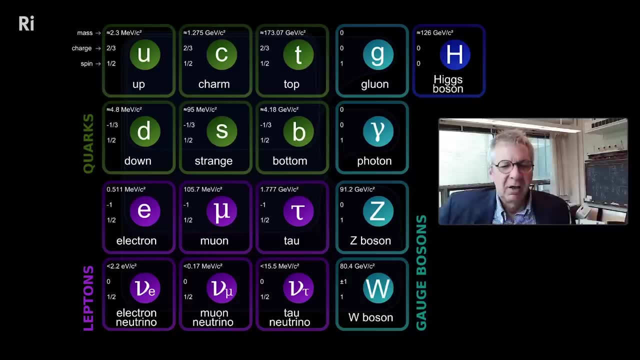 systems were moving very quickly. So, resuming my story in the 1980s, this is a picture of all the particles that we now know make up this model. that we have Shown in green are the quarks. Those are particles that bind together to make the nucleus. 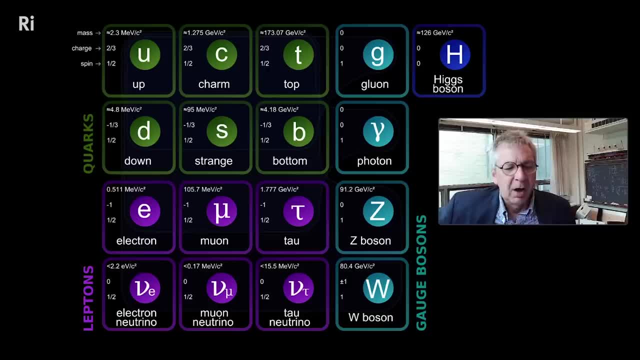 Shown in blue are purple. Those are lighter particles called leptons, And you'll probably recognize from chemistry the electron. And the electron has two cousins, the mu and the tau, And then at the bottom are neutrinos, which we'll come back to in a minute. 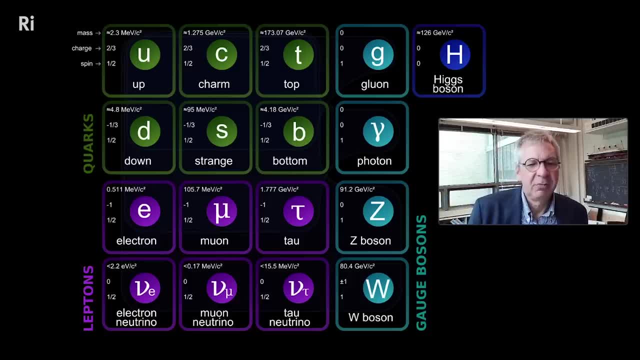 So the purple and green particles, those 12 particles, are all matter particles And everything in the universe is made up of those particles And really only the up and down quarks which make protons and neutrons and the electrons. 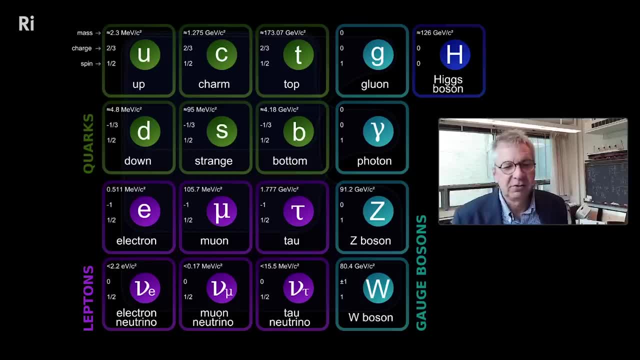 All of the other particles either don't interact, which are the neutrinos, or decay rather quickly to the up and down quarks or the electrons. So those are the matter particles. And then the particles labeled in light blue are the force carriers, the gluon, the photon. 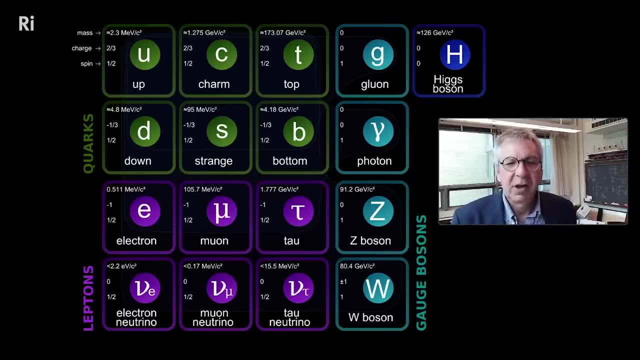 the z and the w, And so, for example, the photon is the thing that makes electric and magnetic fields, And the w and z particles make different fields that make particles decay And the gluons glue up and down quarks together to make neutrons and protons. 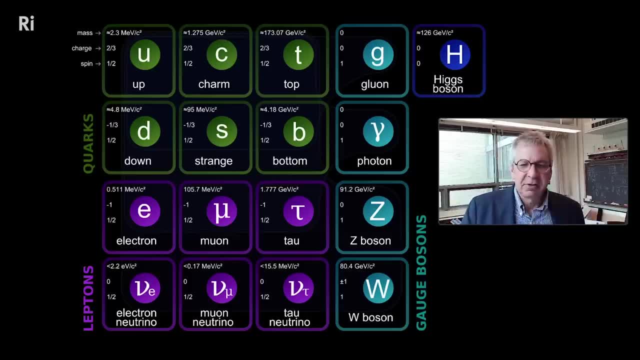 And there was a whole theory checked out in the third decimal place that shows how all of this works. So The way these particles talk to each other, their masses, everything has been experimentally measured very, very well And there's no gaps in the theory. 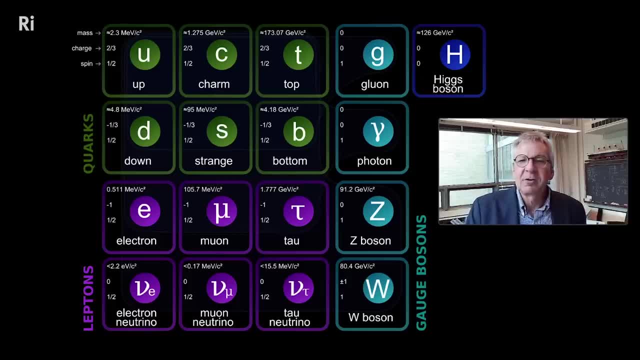 And there's no particle here that could really be a dark matter. particle Off to the right is the one remaining miscreant, which was the Higgs boson. The w and z were the last ones that were discovered in 1983.. 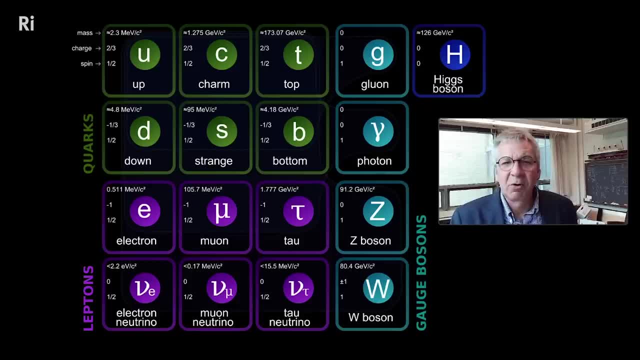 The top quark was 1994 or something, and then the Higgs took about another 20 years and was discovered at CERN in 2012.. These are all the particles that are in this model. They've all been observed, They've all been measured and we know all. 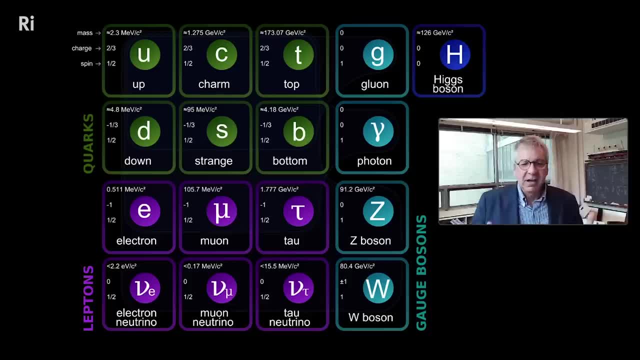 the rules about how they work. So that's why, in the 1990s, people like me thought we really understood everything about the universe, about the matter, About the matter and the universe universe, when in fact, the totality of these particles- 17 particles- comprise about 4%. 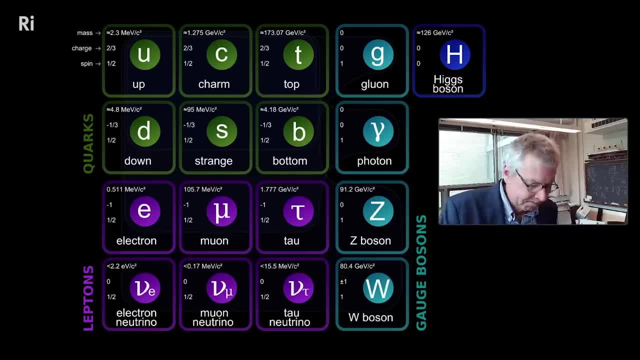 of the mass energy of the universe. Okay, so that's kind of the situation when I showed up. So I started in 1983. This was largely the standard model was largely assembled by then And in 1987 and 88, I was working on my thesis experiment. 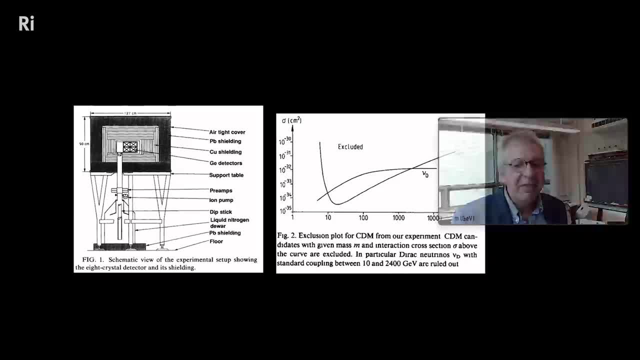 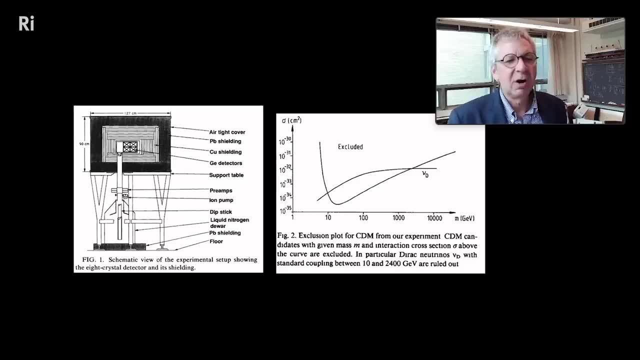 Here's a picture of it. This is actually from my PhD thesis And this was a wonderful experiment because this thing was so simple. It was an experiment to look for a very rare kind of decay, called double beta decay. that took place in the four little boxes with Xs in the very center up on the upper left side. 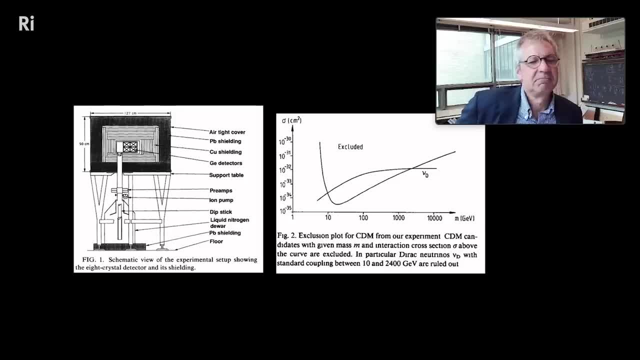 of the left-hand diagram labeled GE detectors. So these were detectors made of germanium And if one of the germanium nuclei decayed in a certain way, there was a very simple electronic circuit that would detect that decay and carry the information out. 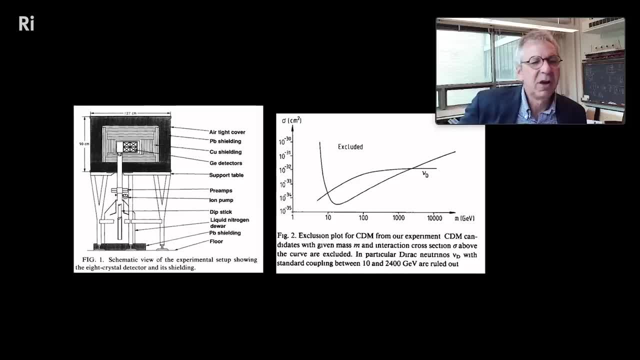 So this was a wonderful project. As a graduate student, I worked on it with just two other people. It went well. It was what I did all the time and they were kind of part-timers. Most of it was. most of the experiment was actually lead and copper. 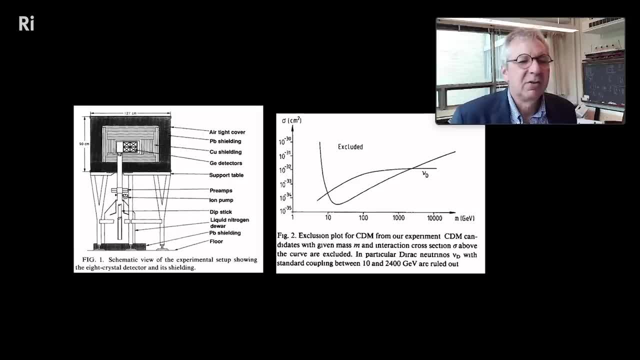 And you can see the source, which were the GE detectors, are surrounded by about 60 centimeters of copper and about 30 centimeters of lead, which we had to stack up by hand, So that whole apparatus is about two meters tall. 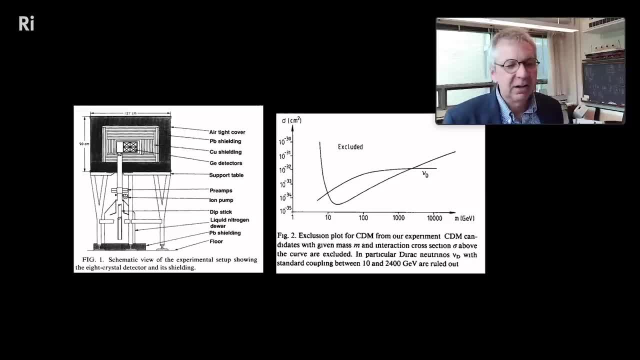 And we had it in the Saint-Gothard road tunnel to protect it against cosmic rays that could make that, could fake germanium decays. And so I was just happily analyzing the data each week from the experiment and working on my thesis. Then I went to a talk at a conference in France. 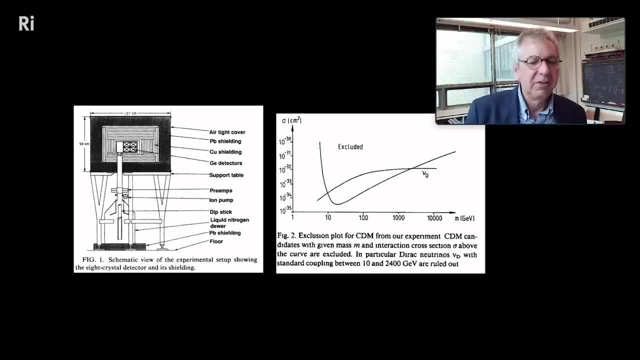 And there a guy named David Spergel, Who was a professor, Who was then at Princeton and now works for the Simons Foundation- He's president of the Simons Foundation- Gave a talk about dark matter, which I had been hearing about, and how dark matter could. 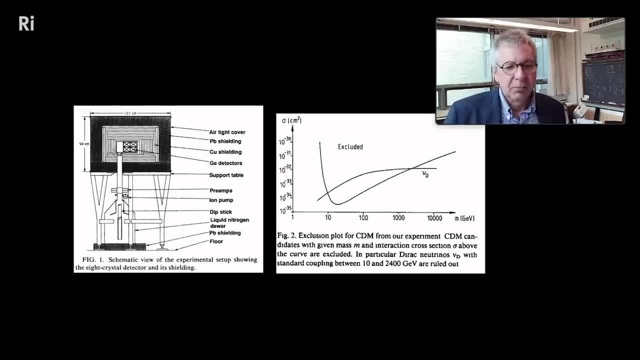 be like a really heavy neutrino. Now, in the previous graph I showed you there were three neutrinos. Those have all been detected and they're very, very light. They weigh much less than an electron. His idea was, If there was another neutrino or something like another neutrino, that was very, very 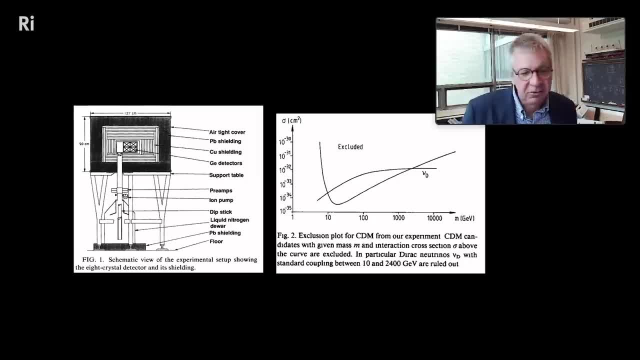 heavy, it wouldn't interact very much, because neutrinos don't interact very much. In fact, you could take a neutrino and you could shoot it through 200 Earths. You line up 200 Earths side by side by side. That neutrino would go through all 200 Earths and probably wouldn't interact. 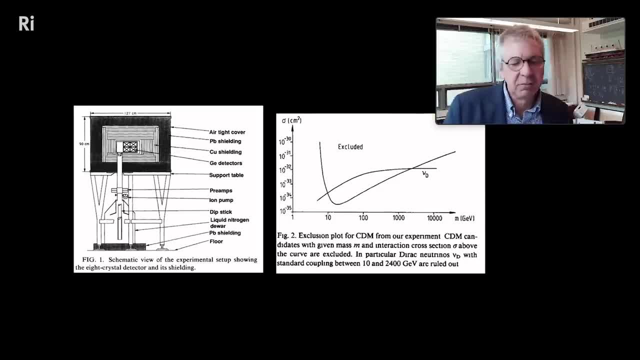 So that's why you'd never detect it. And it's just floating around in space And all it's doing is making the gravitational field we need to explain dark matter. Well, what he said was that every once in a while, one of those neutrinos could bump. 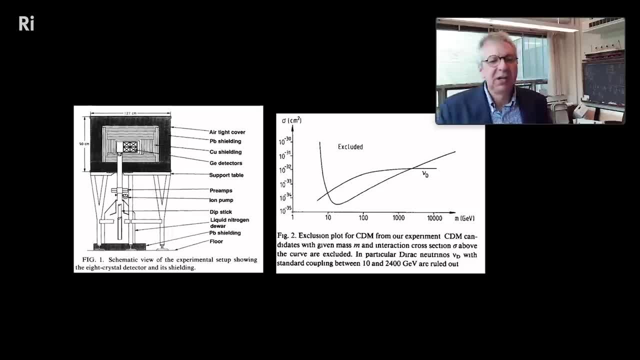 into a germanium atom and leave a little bit of energy that would be recorded in my experiment. So my PhD advisor, Felix Bohm, suggested: Well, I don't know, I don't know, I don't know, You know which I wanted to, like a hole in the head. 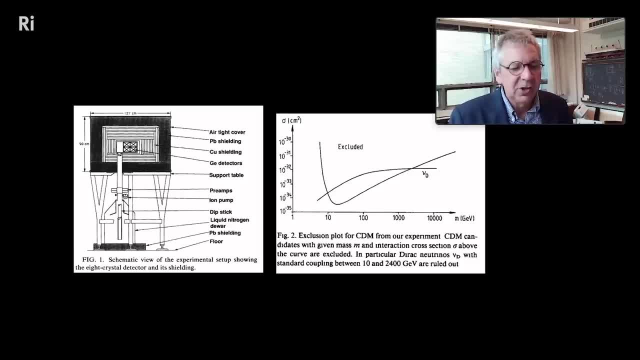 Remember I'm writing my thesis to get out of graduate school- that we make a small change the apparatus and look for dark matter, which we did. We didn't find dark matter, but we did show that dark matter couldn't be a heavy neutrino. 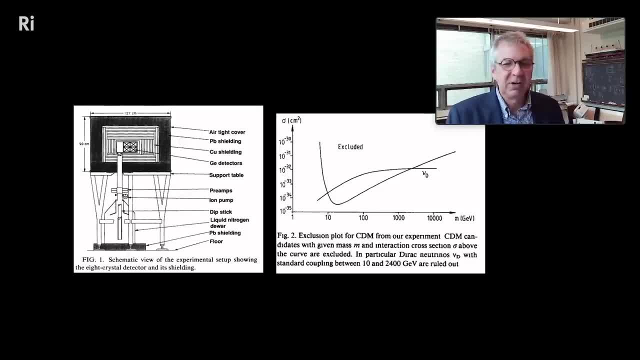 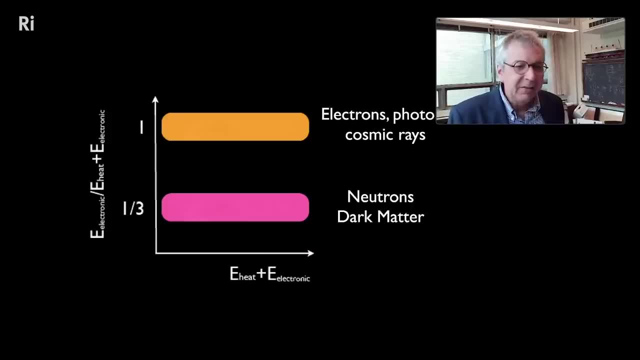 which was an important result, because it had been a heavy neutrino, We'd have seen it, And that's what the plot to the right is showing Right Now. at that same conference, there were a couple of guys who were really working: Bernard. 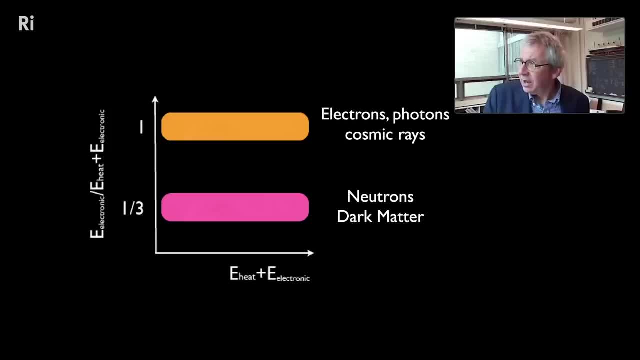 Sadele and David Caldwell, and there was somebody else. They were trying to understand exactly how the energy of the struck germanium got out of the detector, and they found out that if a dark matter particle hit it, a third of the energy would be electronic and two-thirds of the energy would be heat, whereas, if anything, 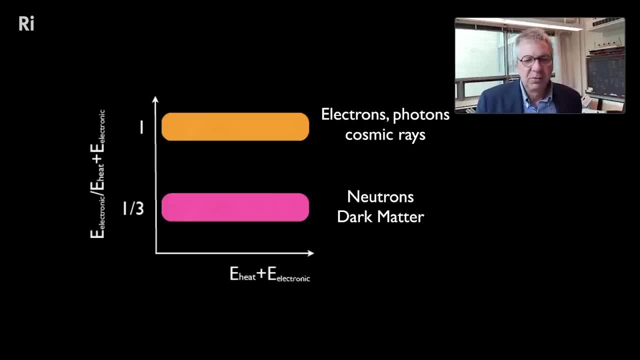 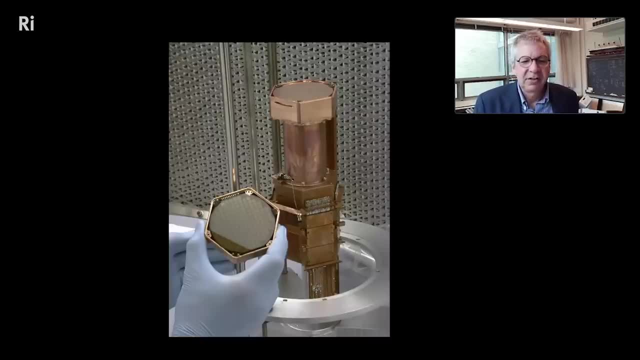 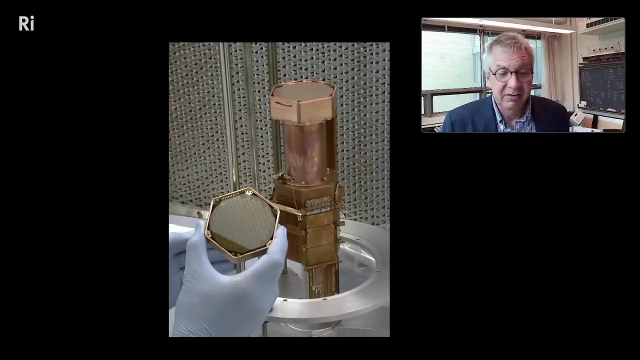 else hit it, all of the energy would be electronic. So they created this marvelous thing which is a detector with thermometers all over it that could tell whether the deposited energy was heat or electronic or both. This was called CDMS. There have been a series of experiments since mine in 1988. 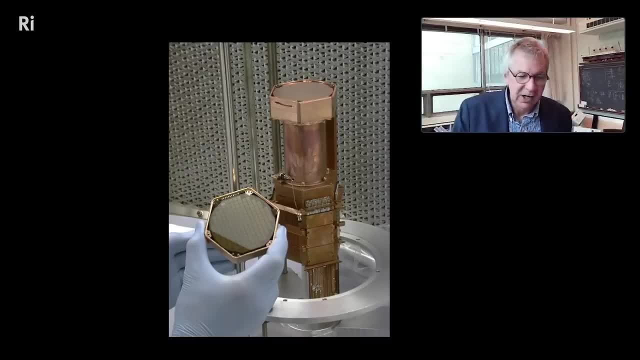 They've gotten bigger. They have this marvelous new technology. the radio purity of the things, which is important for fake signals, got a lot better, to the point where now these experiments are 10 billion times more sensitive than the one I did in 1988.. 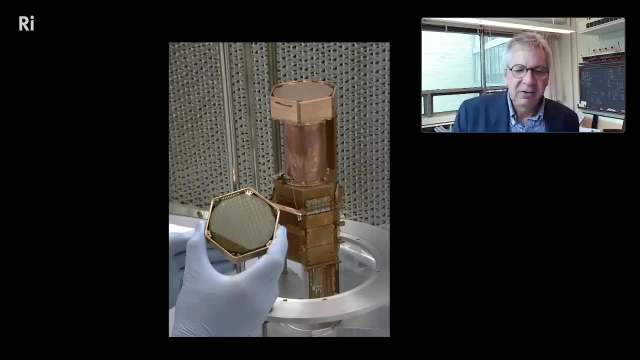 That is an amazing achievement, And what it tells you is that a dark matter particle, if it works like a neutrino, could go through 10 trillion Earths without hitting anything. So these things are very, very hard to detect and have not yet been detected. 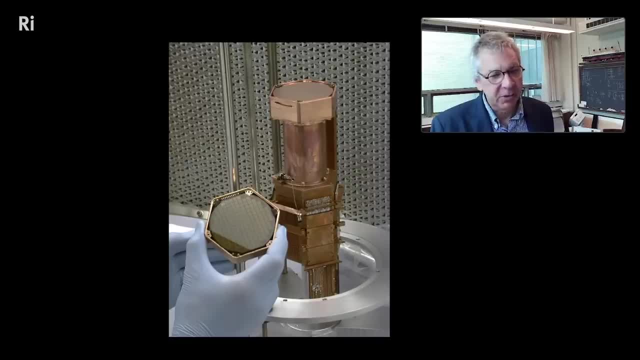 So that's one way of looking for dark matter particles, and this is a specific version of dark matter called the weakly interacting massive particle picture or WIMP, And this is a very specific version of dark matter called the weakly interacting massive particle picture. 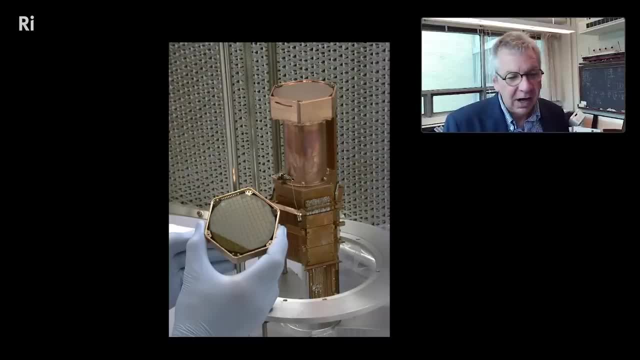 This is a very active area of research. today, My experiment weighed a couple of kilograms. The current experiments weigh many tons. This is just in order to get more things for the dark matter to hit. This is a picture of the accelerator at CERN. 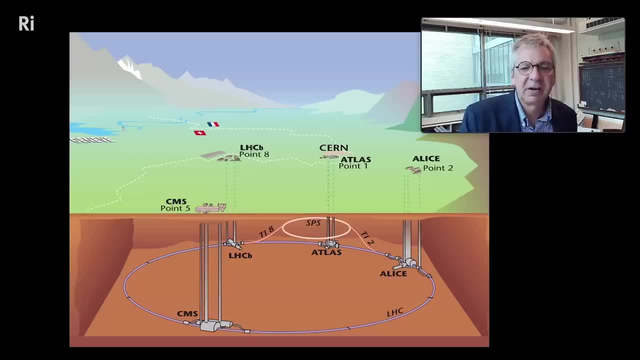 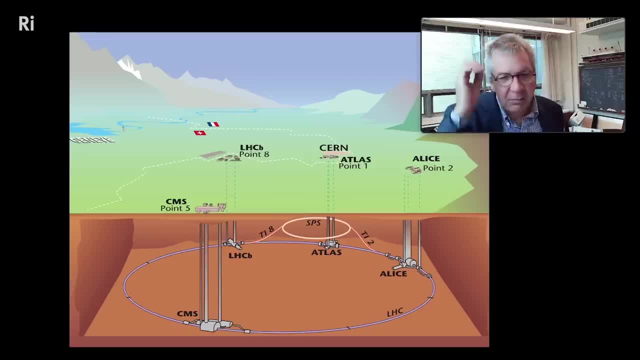 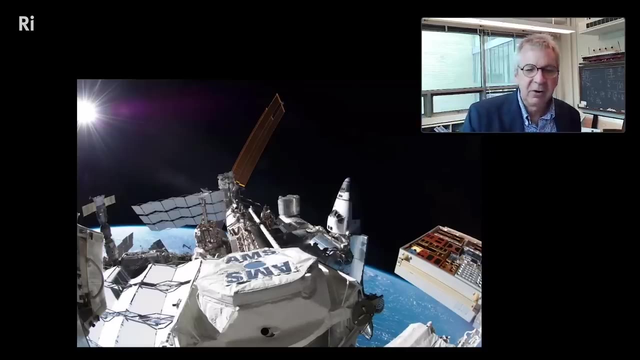 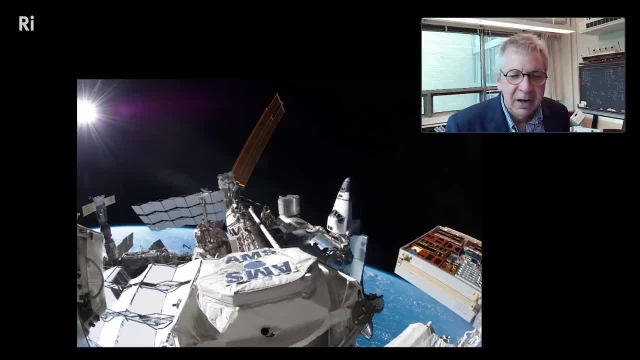 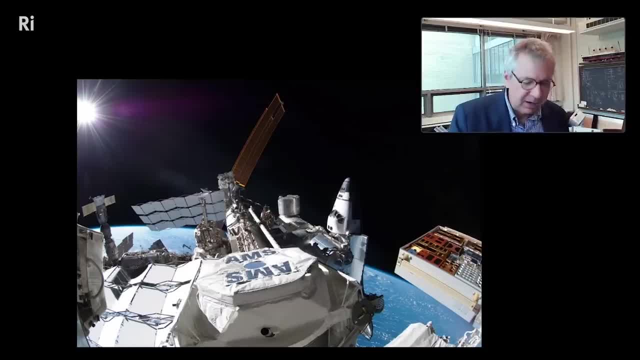 Stay to stay and move to another page. And here now I'm sitting in With the International Space Station. And here now I'm sitting in With the International Space Station measuring cosmic rays. We've learned a lot about cosmic rays, but we haven't detected dark matter. 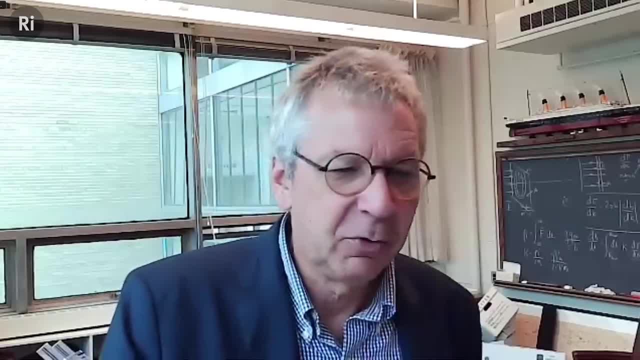 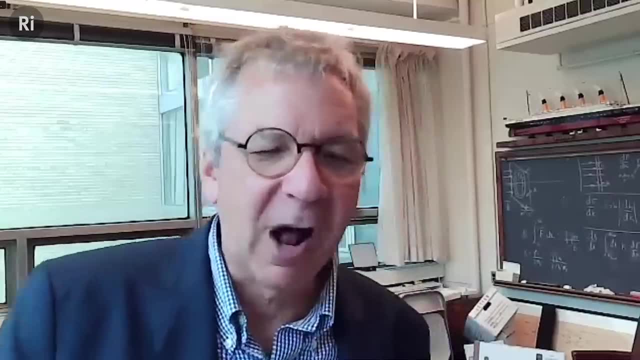 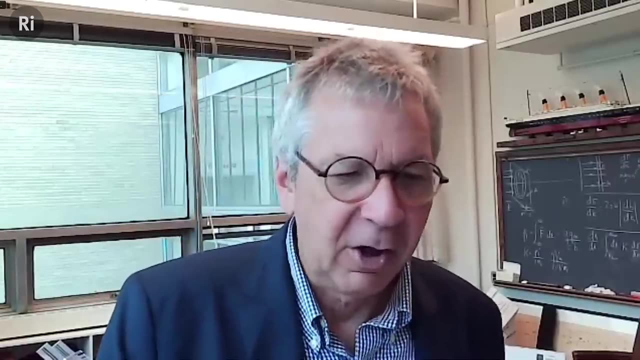 laundry detergent and the creator of the axion theory, Frank Wilczek, called the part of axions because they clean up a problem, a theoretical problem in one of the interactions. Oh and, by the way, axions could also explain dark matter, And if we can share screen, again, this is a 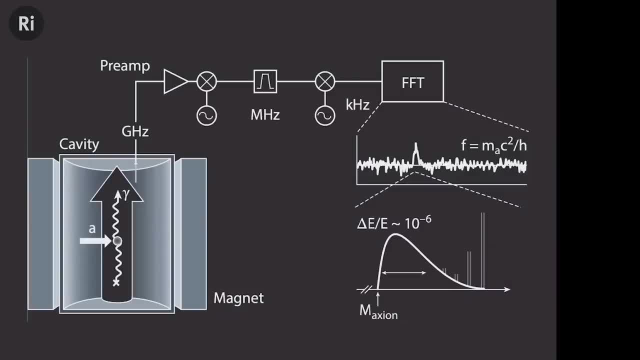 picture of an axion detector that a colleague of mine, Les Rosenberg at University of Washington, built, where the axion labeled A in the little diagram to the left hits a magnetic field photon and turns it into a microwave that's collected with very high precision in this cavity. 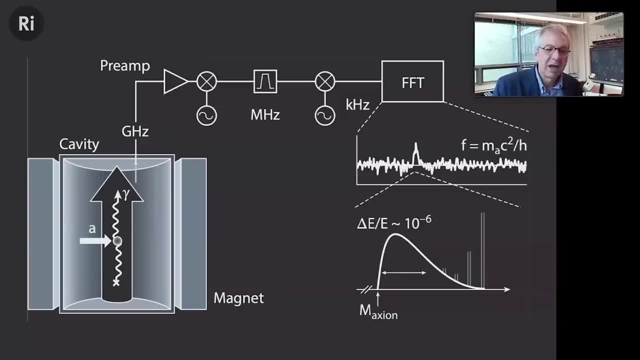 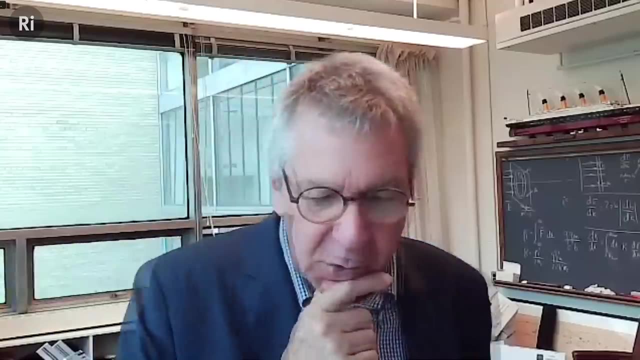 and would indicate the presence of axions. That too has not revealed dark matter. So no WIMPs, no axions. Now, if we go back to 1972, there is a man who's thinking about what the very beginning of the 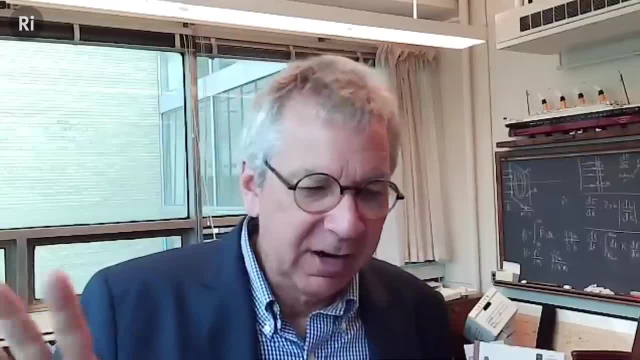 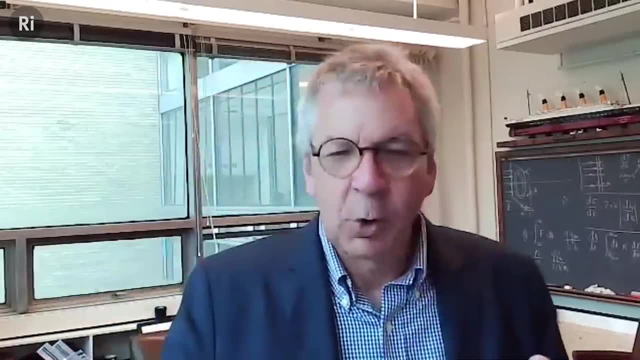 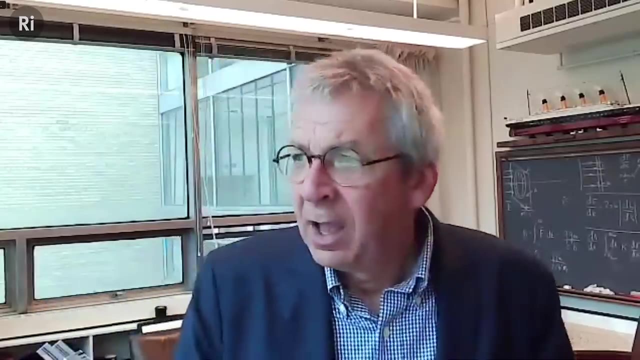 universe would look like. And remember I talked in the very beginning of the universe. there's all this mass around and it's very dense and it's in a regime where quantum mechanics is important. So the density is rattling around and fluctuating and changing And he thought 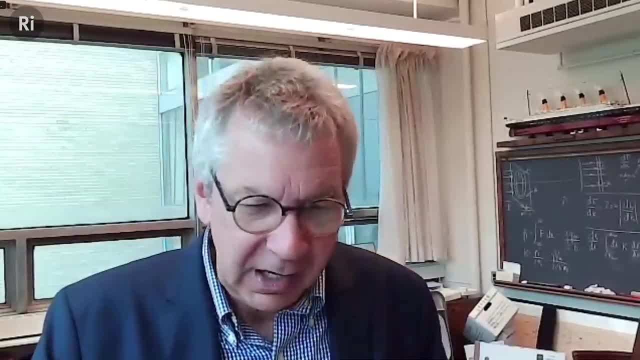 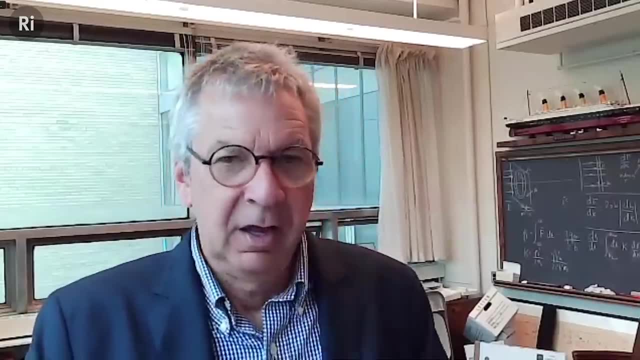 could it be that the density would be high enough to form a black hole? And he did some rough calculations and found out that, yes, they could be a black hole. They collapse into a black hole And in fact, there'd be a lot of 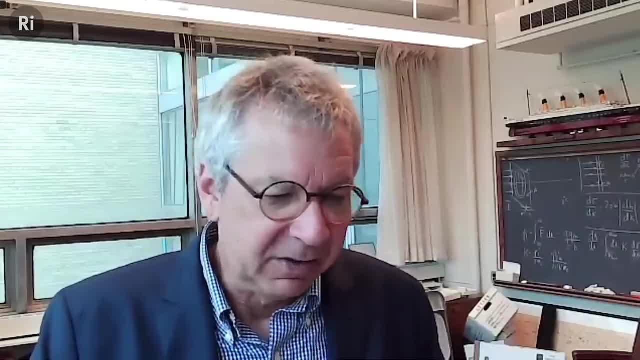 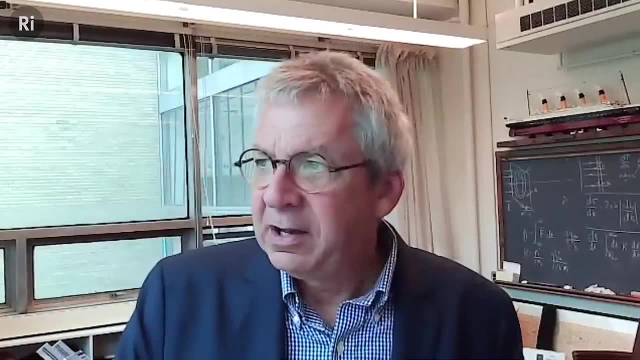 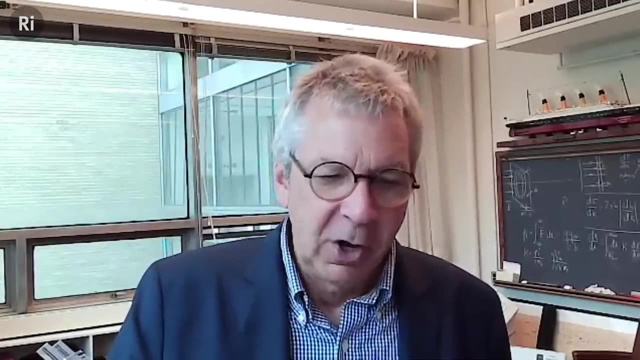 black holes, And there must be some means of getting rid of all those black holes, because we don't see them. That man was Stephen Hawking, And he thought about this problem for a year And in the following year, invented a mechanism by which black holes 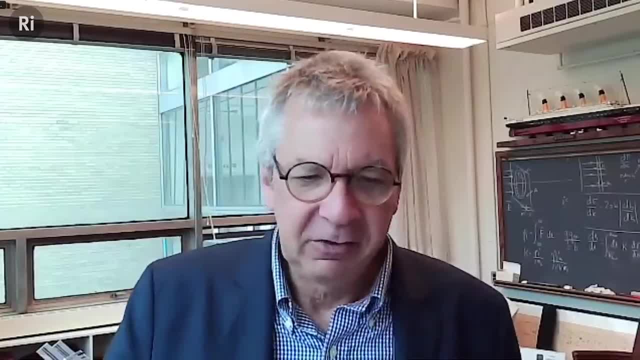 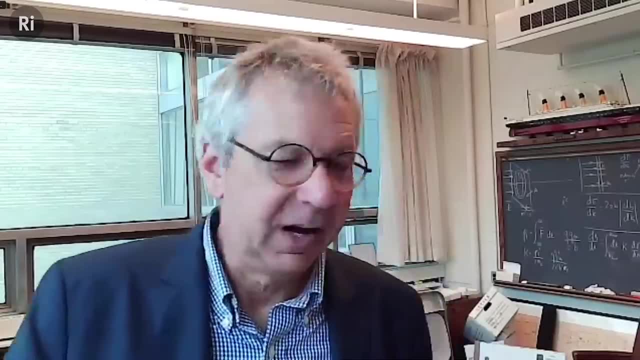 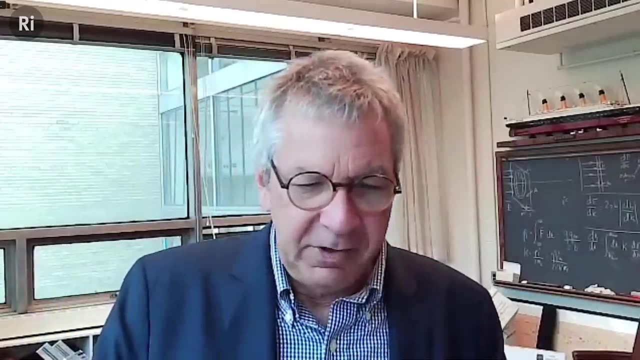 radiate light at a very low level, And this is called Hawking radiation, And this is a remarkable notion because this is the only connection that we have right now between gravity and quantum mechanics. And he developed this theory to get rid of most of the black holes, but not all of them. 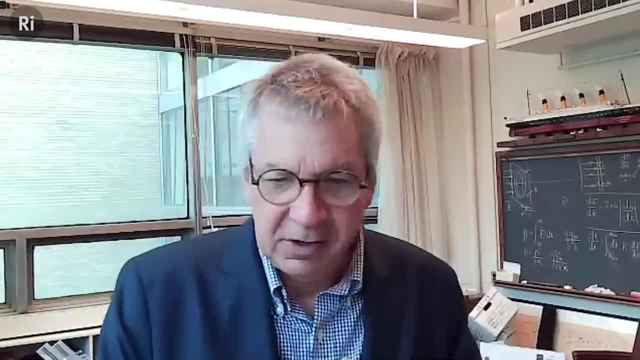 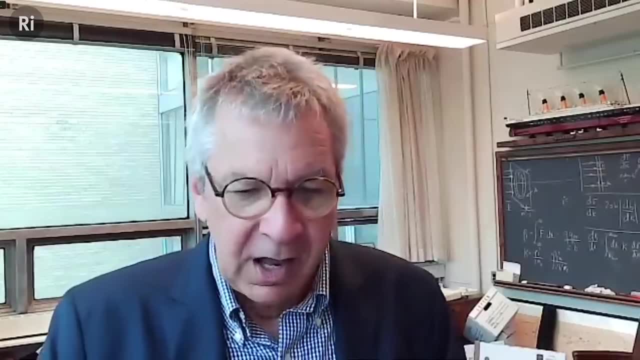 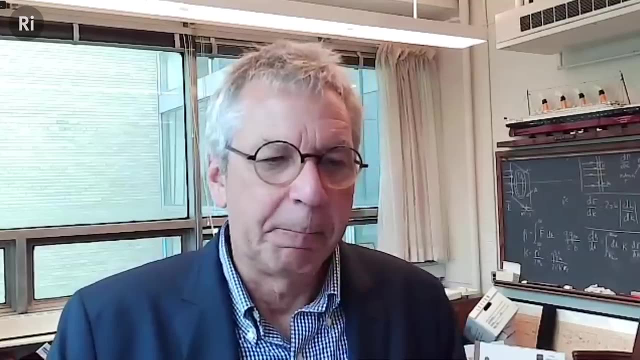 And it could be that there are black holes left over from the Big Bang that would weigh about as much as a comet And be the size of a proton. Those are called primordial black holes, And there are various ways of looking for them, but no result yet. And here, if we can just share screen one more time, 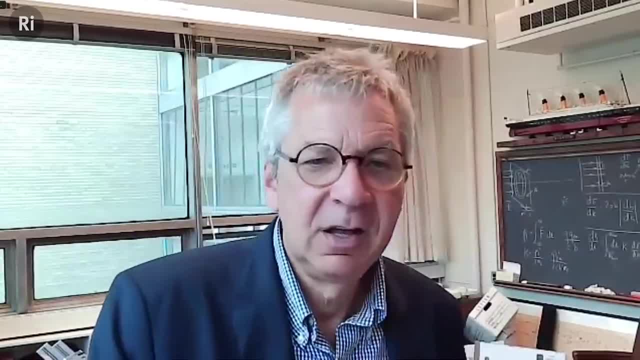 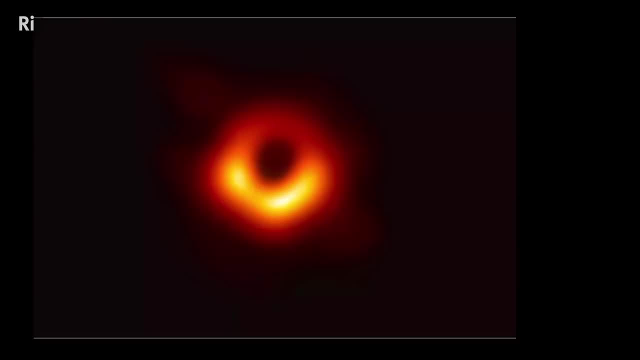 this is a picture that a colleague took the Event Horizon Telescope of the surface of a black hole- And you probably saw this in the newspaper. So weakly interacting massive particles, axions, black holes. Some people have their preferences The story, some people think the story is closed on one or the other, But these are the three.